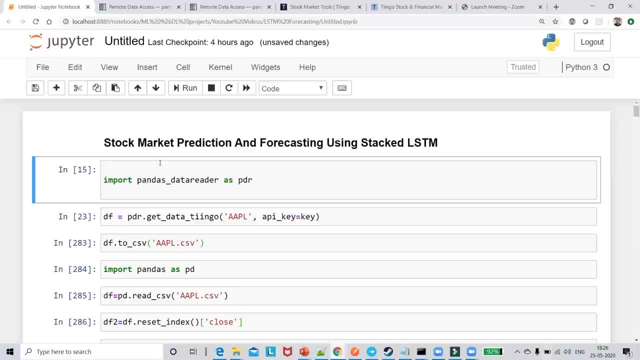 stock market here. I've just tried it to do it by using stacked LSTM itself. I just wanted to show you how we can actually do it. but just don't use this in your real world life so that you put some investment and then after that you lose some of your investment itself. 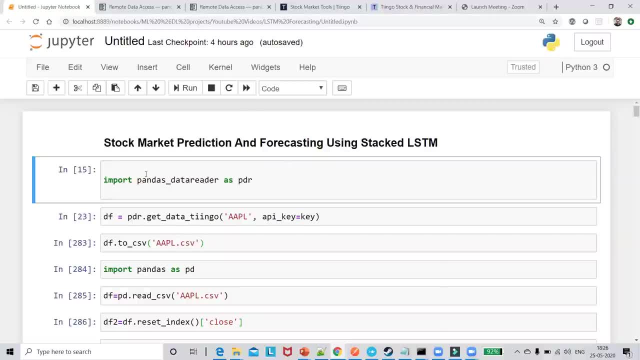 So please don't do that. I request you all. Now let's go ahead and try to see how we are going to do this. Okay, We are going to use stacked LSTM- long short term memory- and probably this video will be more than 20 minutes because I need to explain you step by step. 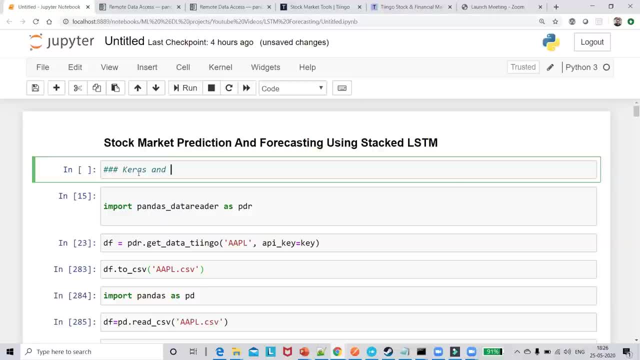 And this I have actually taken care of, Okay, Okay, So I've used this library that used LSTM- long, short term memory, stacked LSTM. I'll tell you how we can actually create a stacked LSTM and we'll actually understand Now the 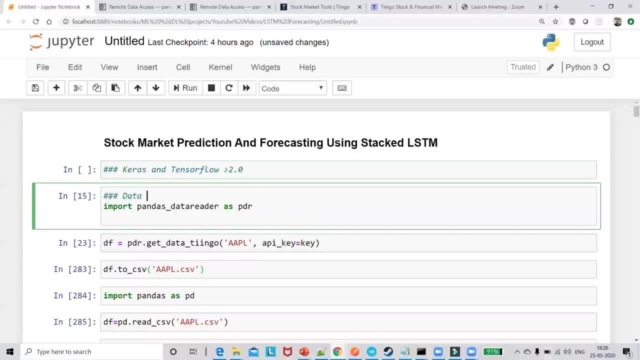 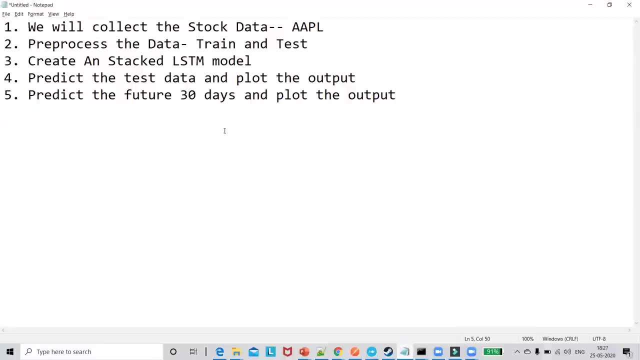 first step is basically the data collection part. guys, Probably for this we need to have some kind of data right, And I'll just show you all the steps that we will be performing. First of all, we'll collect the stock data. In this particular example, I'm taking the 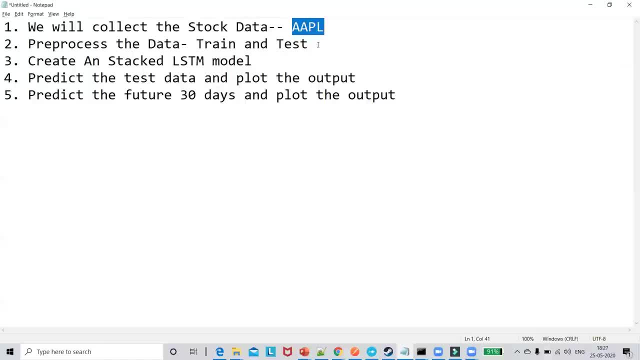 data. The Apple data set Apple company stock prices. you know, from 2015 till today, till 25th. I'll try to take that particular data. Then we'll pre-process the data, That is, divide that particular data into train test. Before doing that, we need to do a lot of pre-processing. 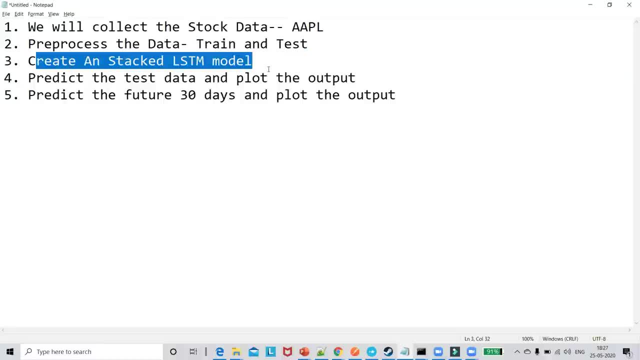 which I'll be explaining. Then we'll create a stacked LSTM model, We'll train it, Then we'll predict the test data and plot the output. Finally, we'll predict the future 30 days, Since that basically means future one month from today's May month. you know, we'll try. 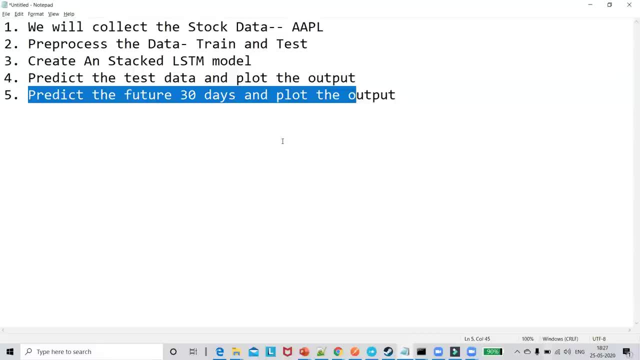 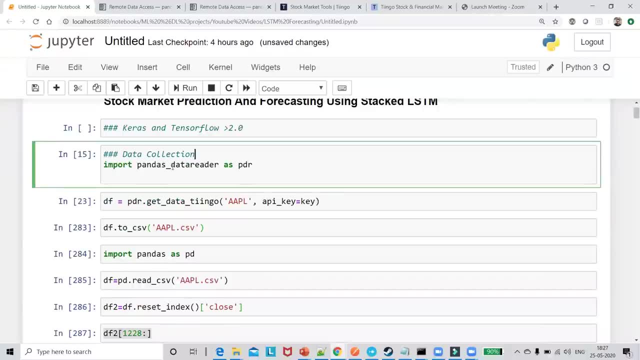 to predict that And I'll try to show you that the output, and we'll plot it also. So let's go ahead with the first step. So here is your data collection strategy. guys, Here I'm going to use a wonderful library which is called as pandas, underscore data reader. 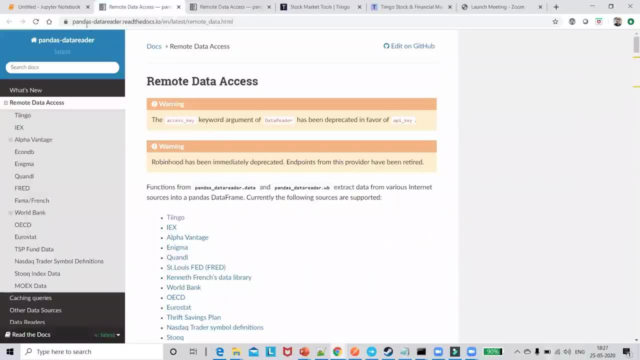 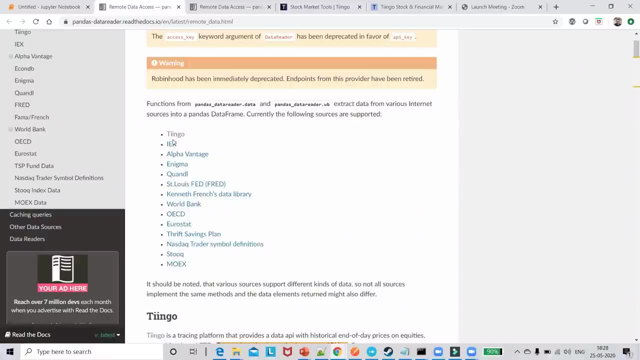 If you really want to see what, in this particular documentation, you can go. regarding pandas data reader, It provides a lot of libraries where you can actually access this kind of data, So currently I've selected Tingo. Okay, In Tingo you can see over here it's pretty. 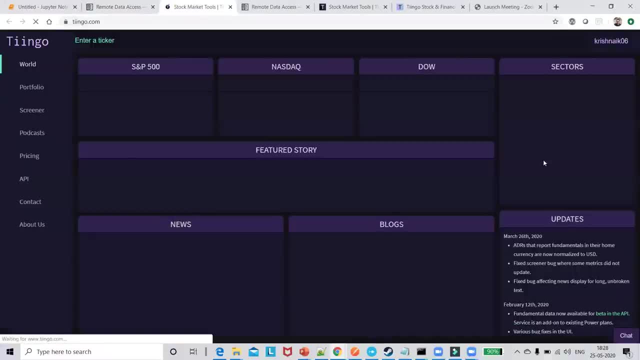 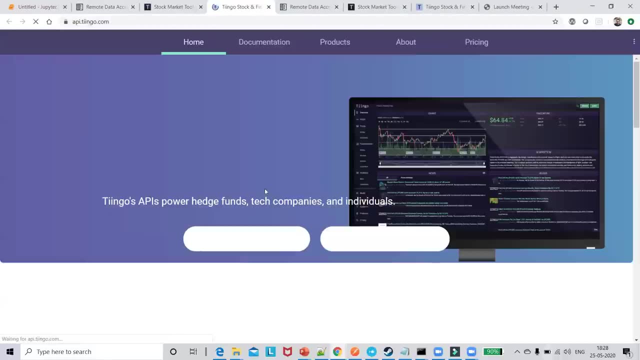 much simple. Just go into the Tingo site, Okay, Just log in. log in inside this or sign up, and then you click on the API part In API. you'll be able to find the key. If you go down in this particular section, in the authentication section, you'll be able to. 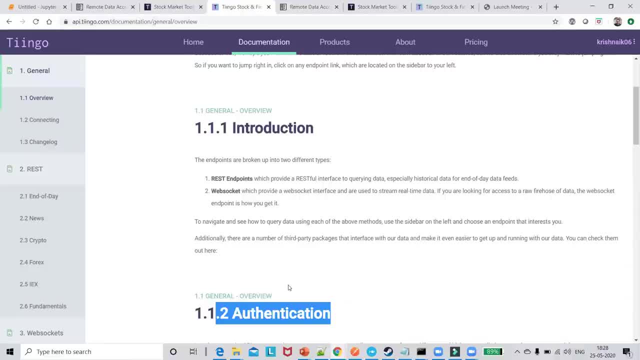 find your own API key. I will not share it with you guys, because I'm going to use that for my personal purpose and trust me for 50,. you can actually request 50 times in a day using this particular API. It is a wonderful way that you can actually collect any amount of data that you like. 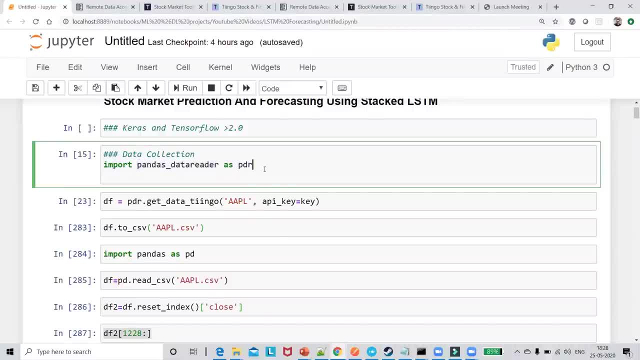 Now I'm going to import pandas data reader as PDR. Then, guys, and this pandas underscore data reader will be already present in your Anaconda environment. Then you have a method which is called as get underscore data, underscore Tingo. Just give the stock price, this particular 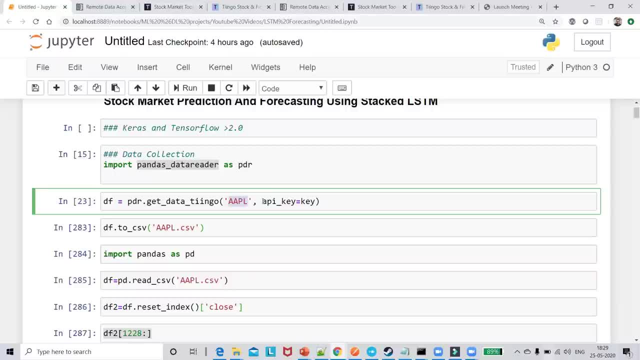 name that is AAPL For Google, you can write GAOG And the another parameter is basically your API underscore key. Okay, so just give this key name. This key name I've already defined over here, but I'll not show it to you guys, So you can execute this particular line and get your value all. 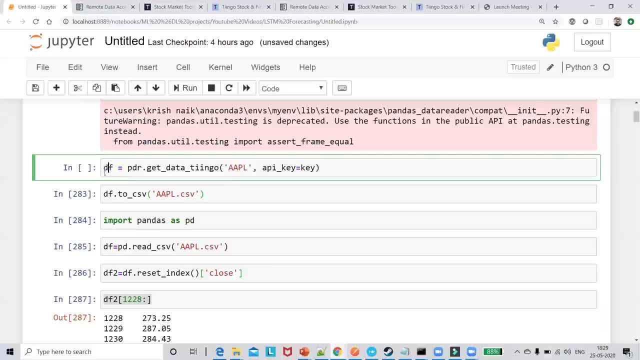 the all, the whole data frame inside your DF variable, Then I will be saving this particular file in csv, As I told you that we just have 50 requests that we can go ahead and hit it. But after this, you can know, you can again re-upload your data set from this applecsv. 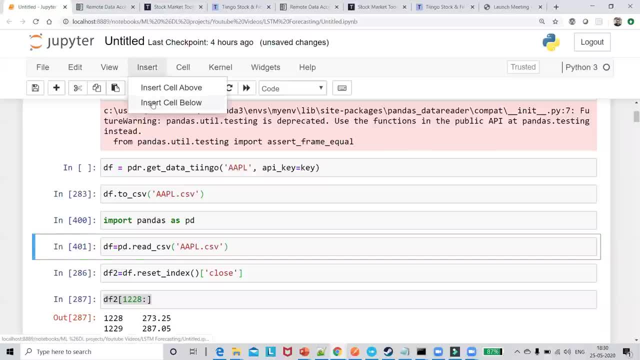 file, which you have actually showed saved right, So below this particular cell, what I'm going to do is I'm going to go ahead and save it, This particular cell. what I'm going to do is that I'm just going to write dfhead and. 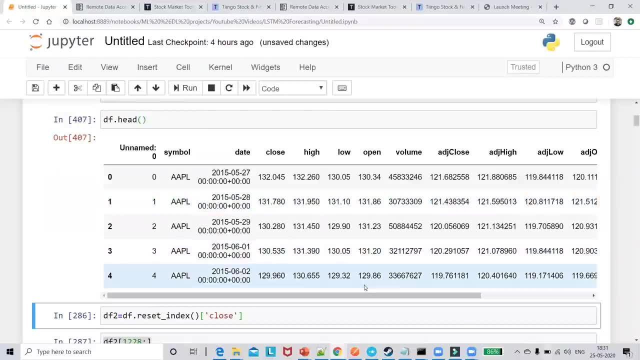 show you how the data set looks like. If you go and see the datahead dfhead, you'll be able to see a lot of features like date- close- high, low, open volume adjust adjusted- close adjusted- close adjusted- high adjusted. 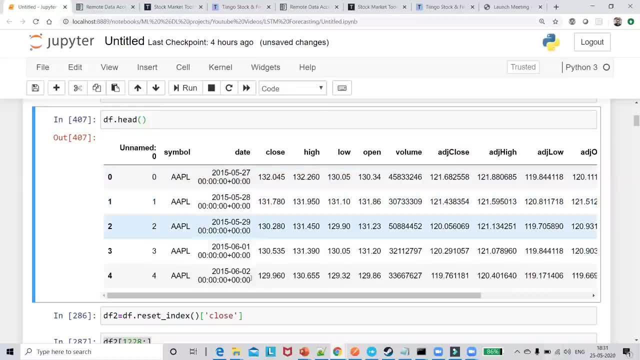 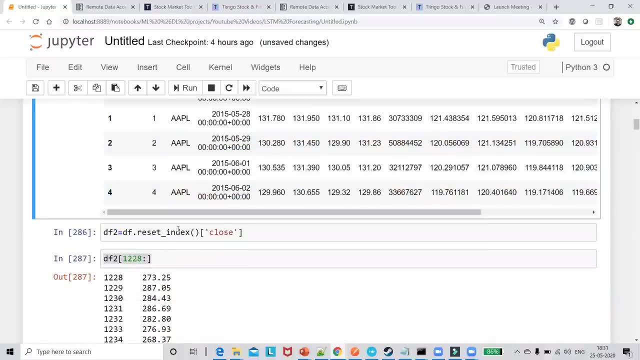 low and many of them. You can take one of them: either close or high. In this particular example, I've just taken high. If you want to see from what date it is, we are having the date from 2015.. And if I go, 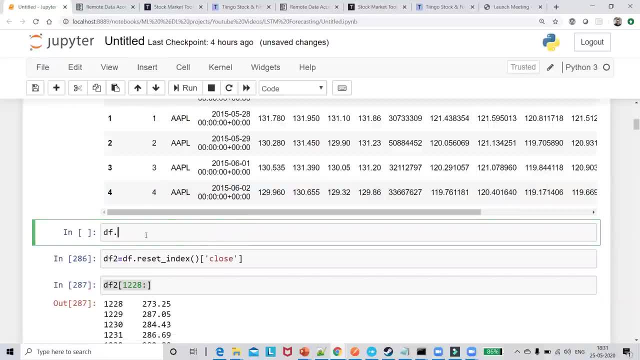 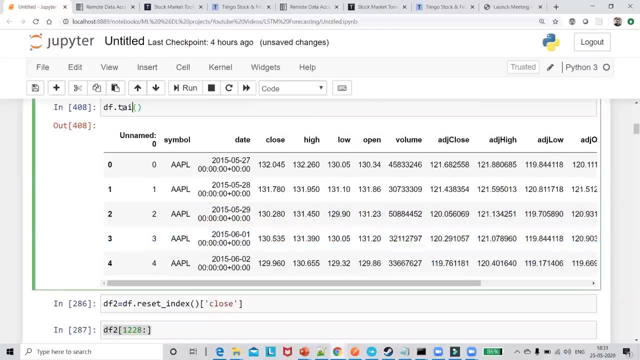 and see the tail of the data set. I'm going to go ahead and save it. I'm going to save the tail of this particular dfhead. You'll be able to see that I'm having this sorry dot tail. If I make it dot tail, then 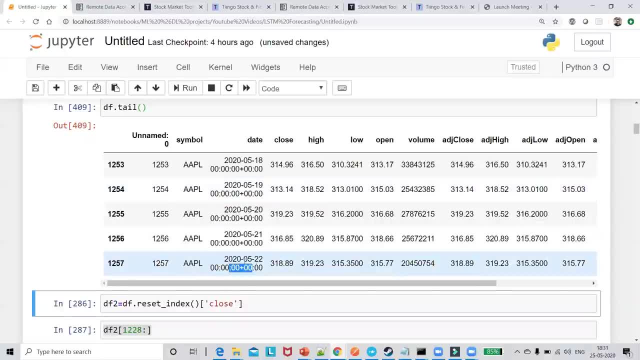 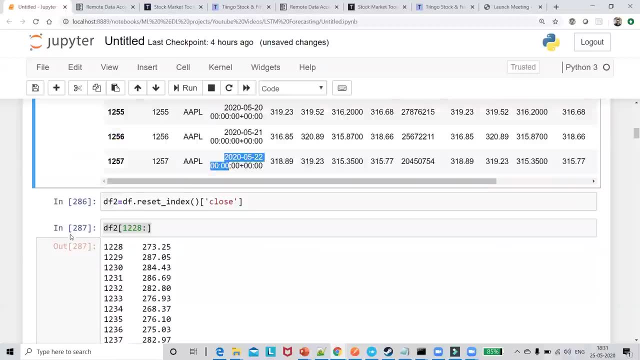 I will basically be having from till 22nd May. okay, So I have the data till 22nd May 2020 for the Apple stock price. Now, what I'm going to do is that, quickly, I'm going to take this close column. okay, I'm going to take this. 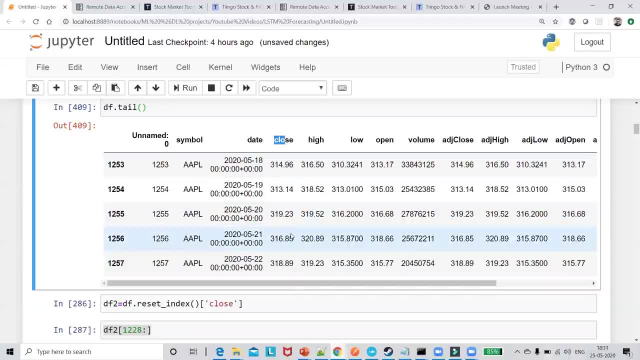 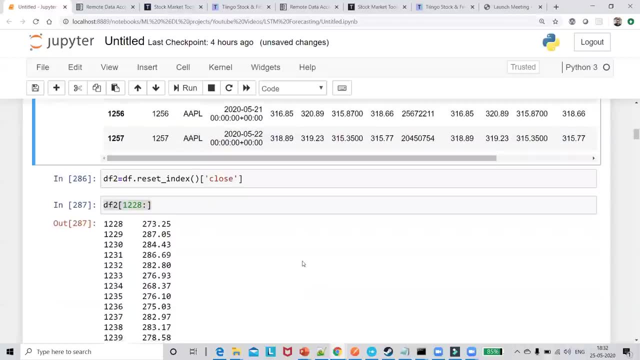 close column and for this particular price, we'll be doing the stock prediction. You can also be able to do for other by using the same strategy and method. okay, So let's go ahead and try to quickly show you how we can actually do this. 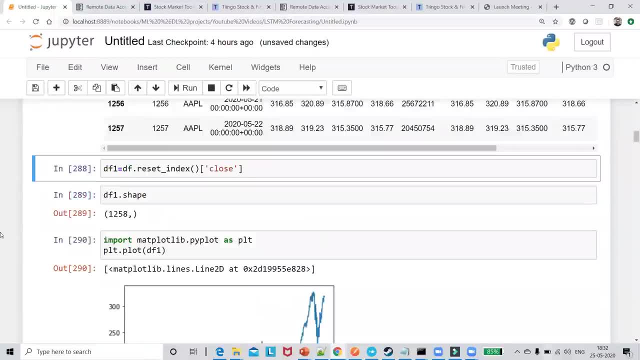 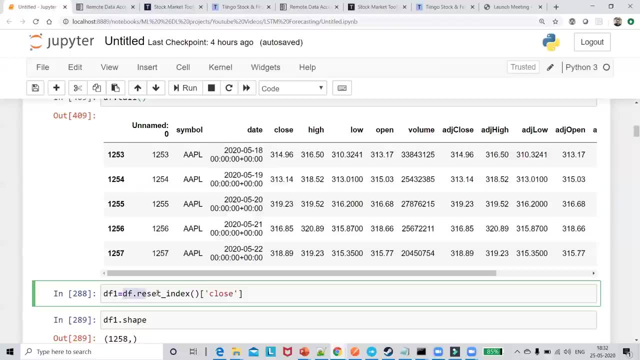 Till then I'll just delete this cell because we don't require it. Okay, Now what I'm going to do is that, first of all, I just want to pick up this close column, right, So for this I'm writing dfresetindex. If I do reset index, that basically means all this particular value. 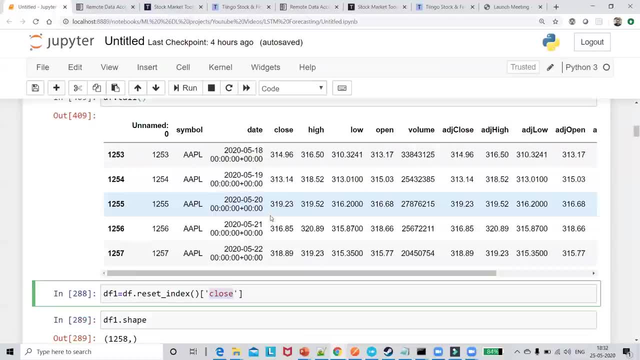 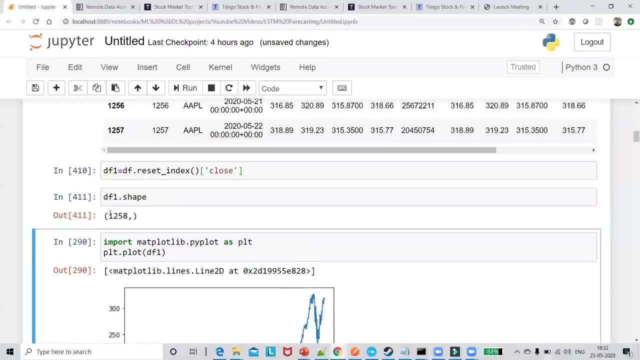 will be going inside this And then I'm just going to take the close column. Okay, So by this I will be able to get all my close values in df1.. So if I go and see the shape, it is having 1,, 2,, 5,, 8 records, Okay. So if you want to really see the df1,. 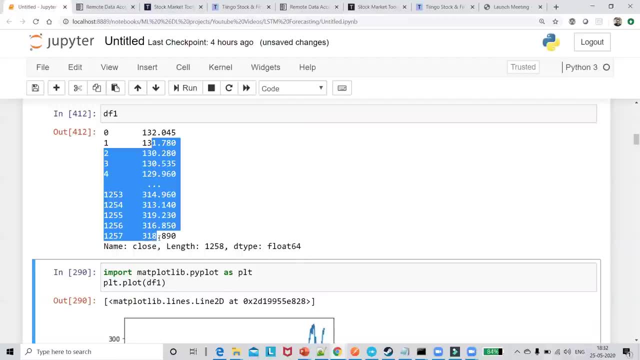 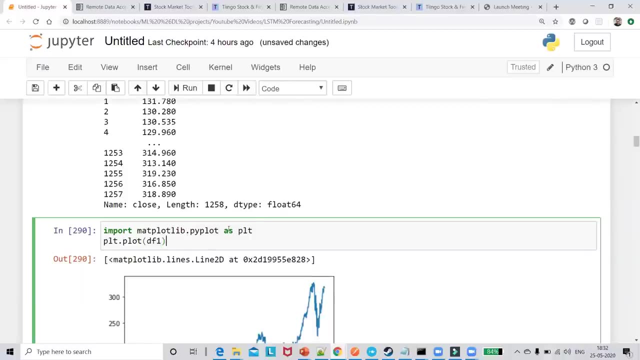 I'm having these values like this. You can see that it is increasing as we go ahead till 1,, 2,, 5,, 7, right, If you really want to plot this particular data frame also, you can use matplotlibpyplot as plt and just use pltplot df1.. So here you can see that this is how. 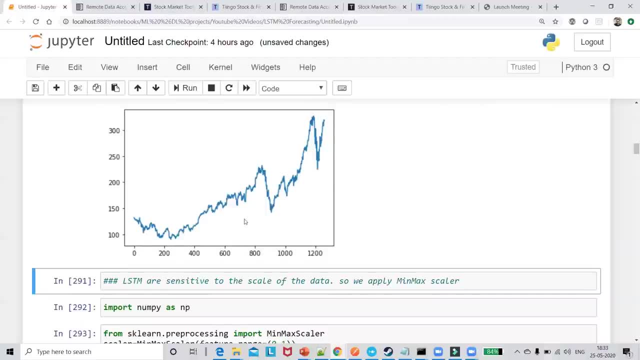 you are plotted. This is what your stock price looks like. you know, from 2015 till 2020, right? So this is how your stock price is having the movement. It has both up and down movement. So let's see how we can actually solve this particular problem. 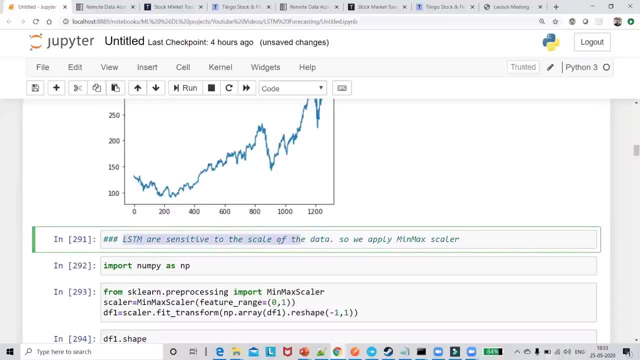 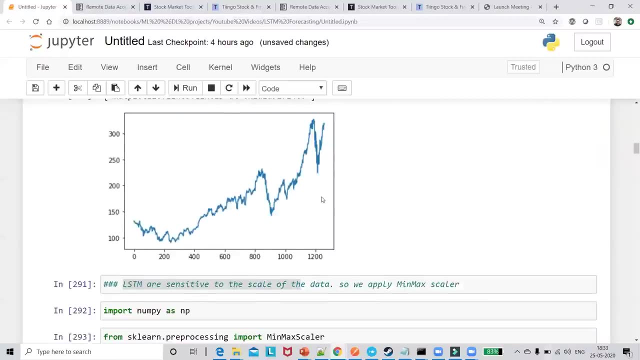 Now, one thing that you need to note is, guys, LSTM are very, very much sensitive to the scale of the data. Now, this particular data, this value, is in some kind of scale, So we should always try to transform this particular value. In this particular example, we are 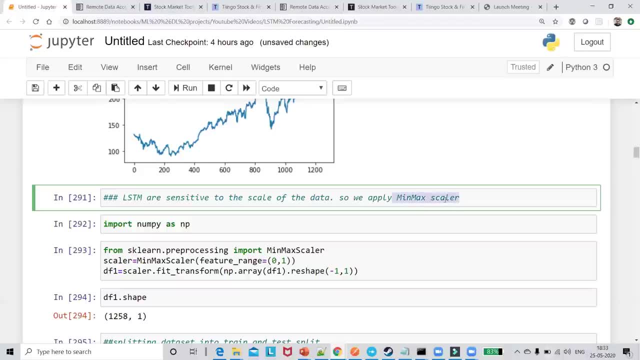 going to take minmax scalar where we'll be transforming our values between zero to one. So for this I'm going to import numpy and I'm going to say from a scale on dot preprocessing, import minmax scalar. In the minmax scalar I'm going to take a feature range between 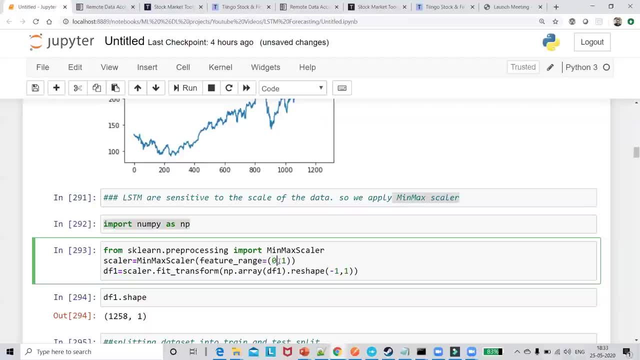 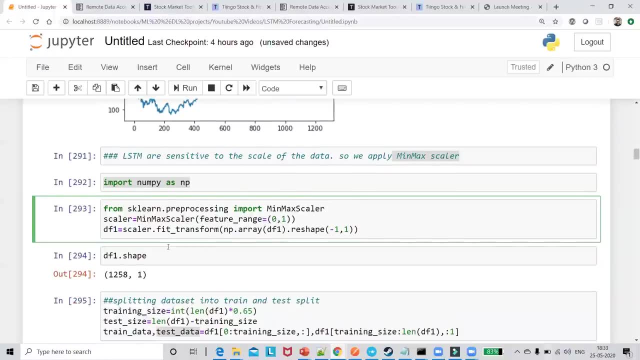 zero comma one. Okay, So this: this is the value that you need to give when you want to scale down between zero comma one. Suppose you want to scale down to the minus one comma one, you can give that value also After that. I'm saying that scalar dot fit underscore. 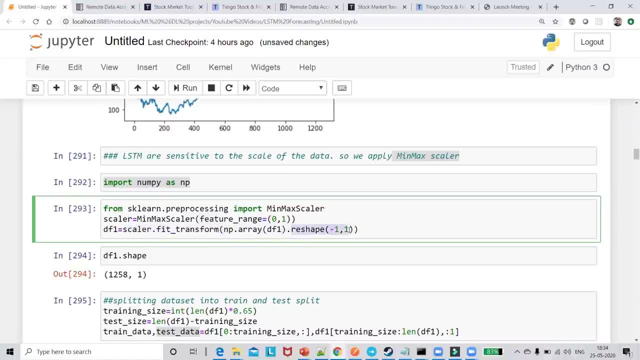 transform np. dot array, df one, dot reshape minus one comma one. You have to do this particular step, guys, so that you'll be able to provide this particular input to fit underscore transform. Now let me quickly, first of all, show you how your df one looks like, you know. so your 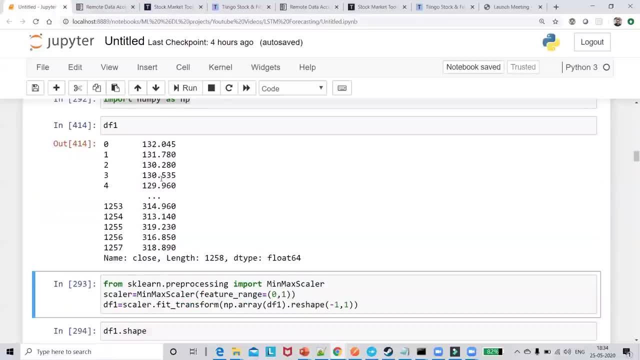 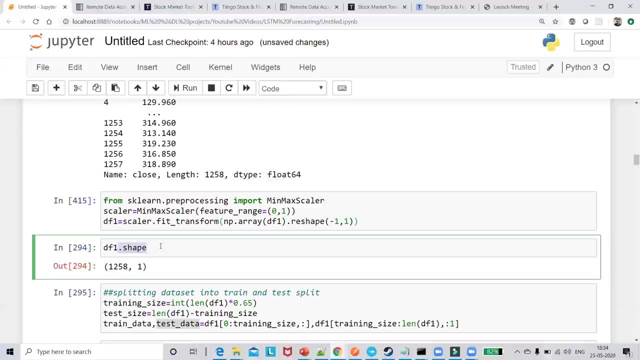 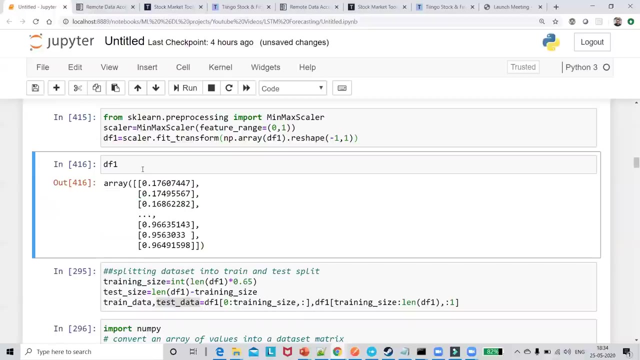 df one has values like this: 132,, 131,, right- All these values. Now, after executing this step, you will be able to see your df one will be now converted into an array and you can see it is now having values between zero to one. Okay, So it has got transformed between 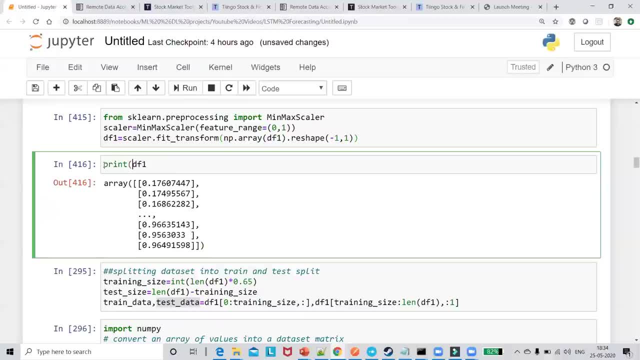 zero to one. Suppose, if I try to print this value, let's see, you'll be able to see, uh, all these particular values that are there- And remember, this is between zero to one, all these values that you can actually see away. Now the most important step right over: 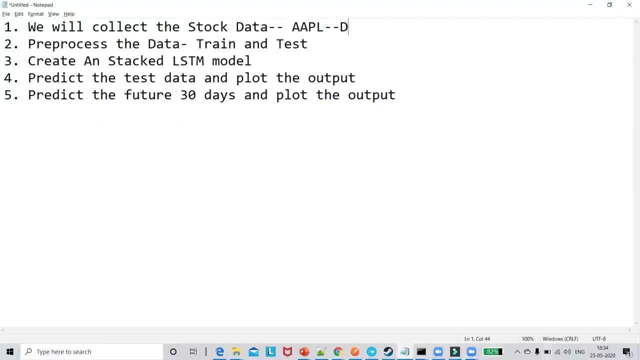 here. I told you that we have done this particular step. I'm just going to write: done, Okay, Now we need to pre-process the data before that, So let's go and do the train test plate Now. one, one important thing: whenever you're. 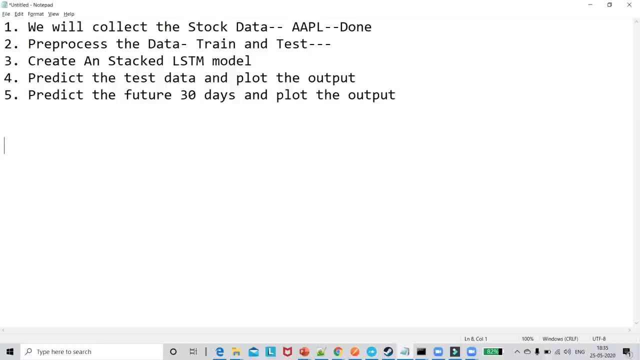 dealing with time series data. guys understand, suppose for the first day the stock price was $120. Then it came to one 30, then it came to one 25, one 40. I'm just taking an example, guys. Okay, So one 51, 60, suppose. this many information I have right now, right. 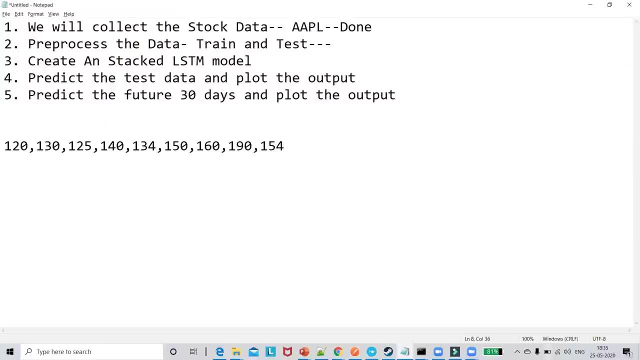 Now, first step: what I, what you always have to do during the train test, Is that there are various ways of doing trend test right. One is cross validation- Okay. One is directly by using some random seed- Okay, But this all methods, if I talk about. 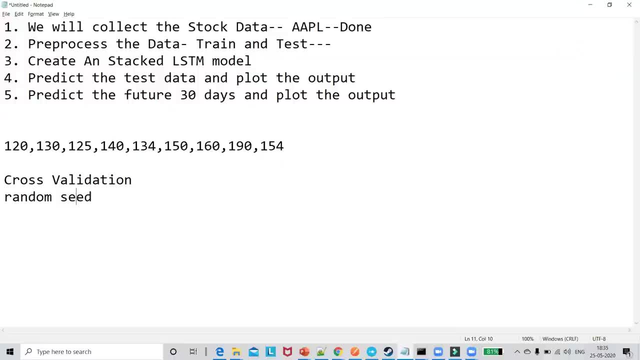 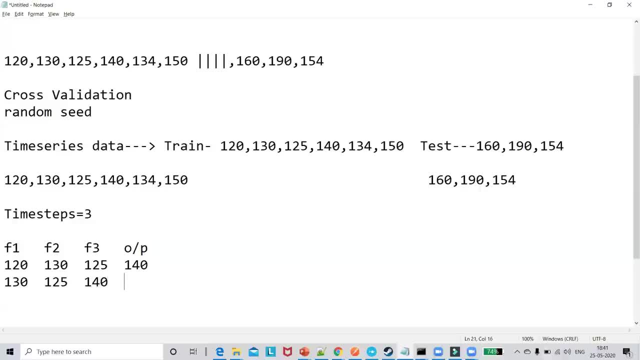 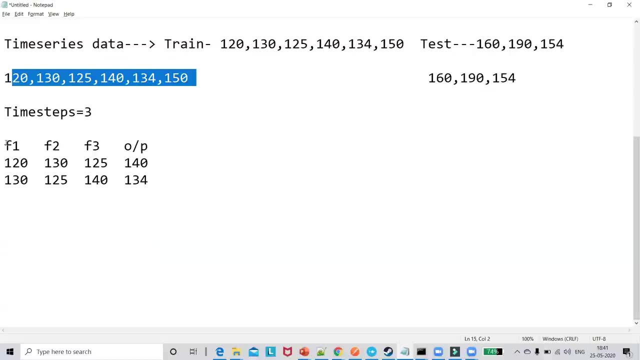 way. So how do we divide the data set in a different way? So how do we divide the data? and then my output actually should be 134. so we will be actually doing like this. we'll convert this whole data set and convert this into our training. this will this. f1, f2, f3 will be my. 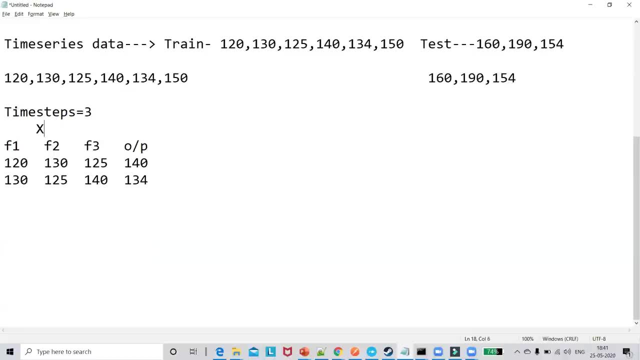 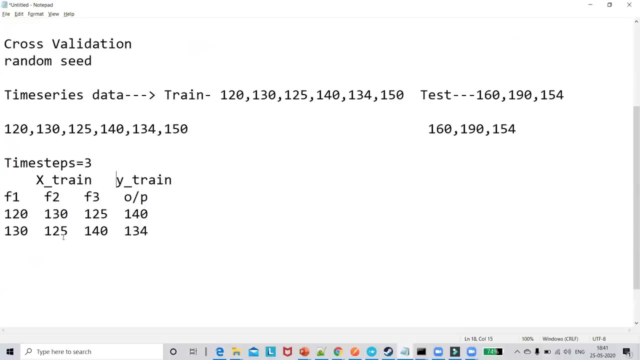 extreme, so i'm just going to write it down over here. so this will be actually my extreme and this will be my white. pretty much simple, right. so these are my two data set. you can clearly see that independent features, dependent features. now, similarly, this is my independent dependent. 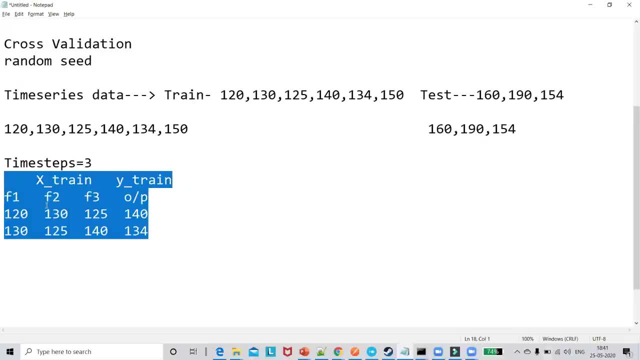 feature. now, considering this data, i will try to use it in my lstm model to train it. you know, then, for the test data also, i have to do this in this way itself, in this similar way. i need to make this particular split right. we suppose i have some more elements like 160. 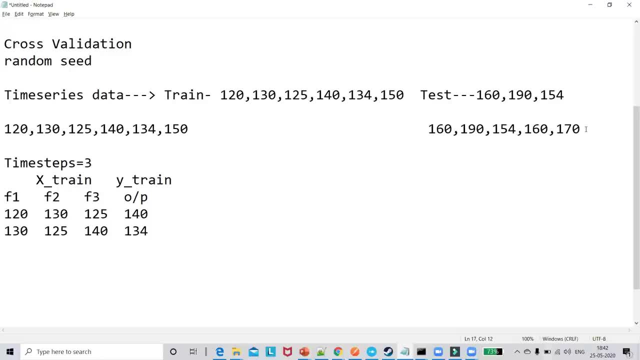 170. okay, i've just taken some example, guys, so please bear with me in this. so, okay, here also i have to do the same processing. that is f1, f3, right, and here this will be my output. remember, whatever output this is, this is basically my y underscore test. okay, and this actually is my y underscore. 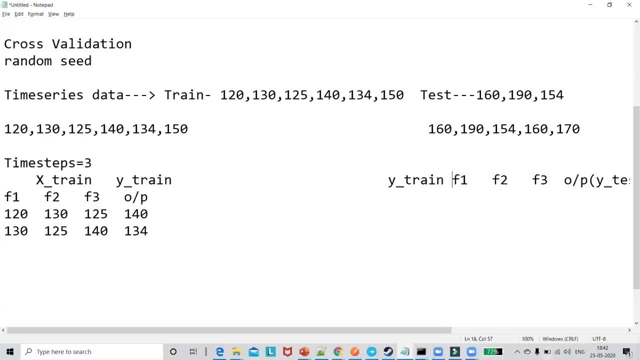 this is my y underscore train, right? so i have all this particular information clearly given to me in this particular way. so i have all this particular information clearly given to you. okay, now, similarly what i'm going to do, i'm going to write 160 over here. you will be. 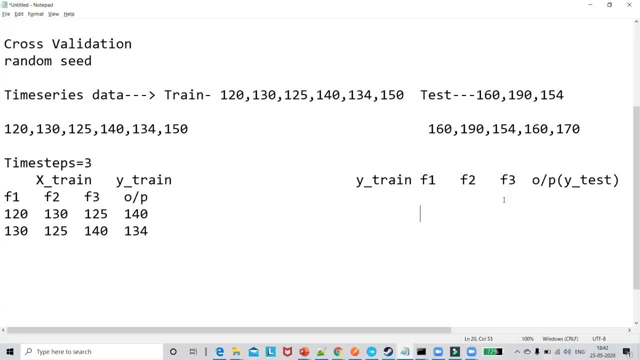 able to see it. i'll be writing 160 first. my data pre-processing will have 160 over here, then 190, then 154, you know, and then my output will be 160, right? similarly, similarly, you can see that i've taken the first four elements. now, in the next element, again, what will happen? 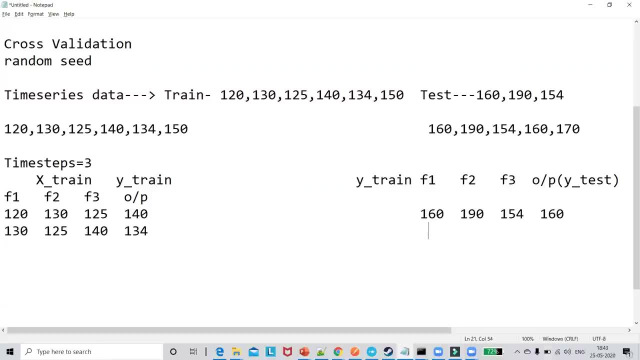 if i, if i see over here, it will just go over here. it will take the next three elements: 190, 154 and 160. the next output for this is: you can see 170. so this will basically be my white test. then what i'll do is that after i train my lstm model with this training data set, i will take 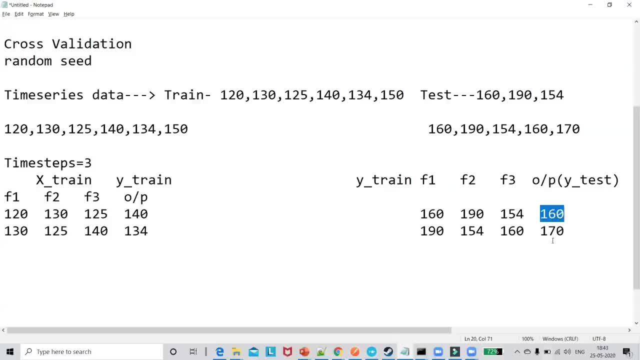 this test data set and predict it and then try to compare with my y underscore test and then we will be seeing that how good the accuracy is coming, how good the- uh, you know the forecasting is actually coming. so we have understood this. the data pre-processing is pretty much simple, guys. i. 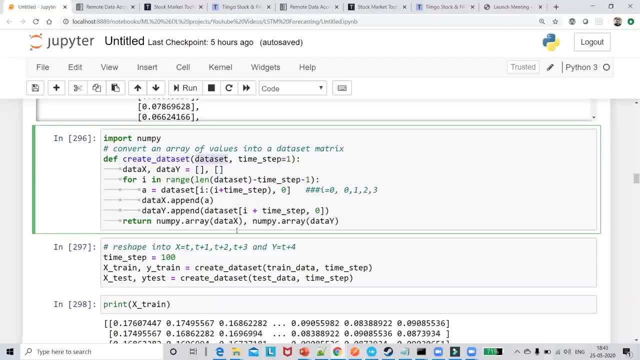 have created a map to this. data pre-processing is actually pretty much simple, guys. i have created a method which is called as create data set. here we actually take the data set. then under timestamp in the timestamp by default, whatever values are giving like hundred, it will be taking hundred timestamp, like this here. in this case, it 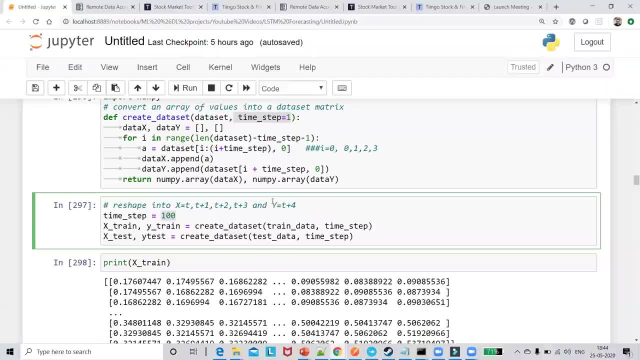 is three timestamp, right. so here it will be taking a hundred timestamp and remember the more better you have a timestamp value. this is again a hyperparameter tuning technique which we will be selecting those timestamp values. so inside this particular method, that is, create data, set what we are doing first. 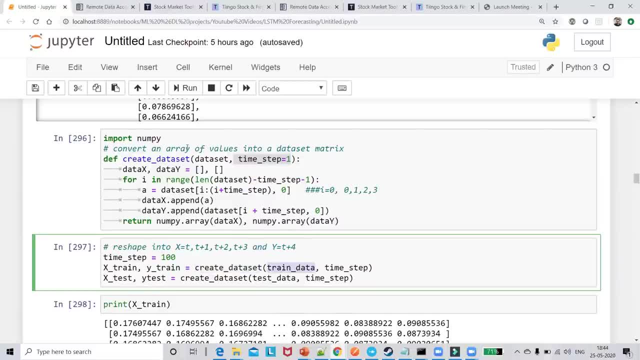 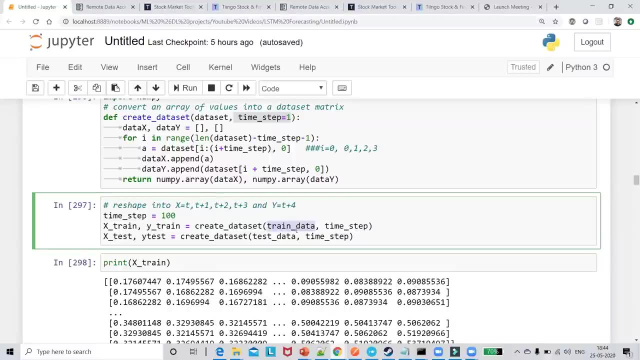 of all, we give our training data. similarly, how we got, we divided the training and test data on the top right, like how we, how we explained over here. now, for this train data, I am saying that you know, take the timestamp value as hundred. okay, make your data set as X and Y in this particular manner. this is the 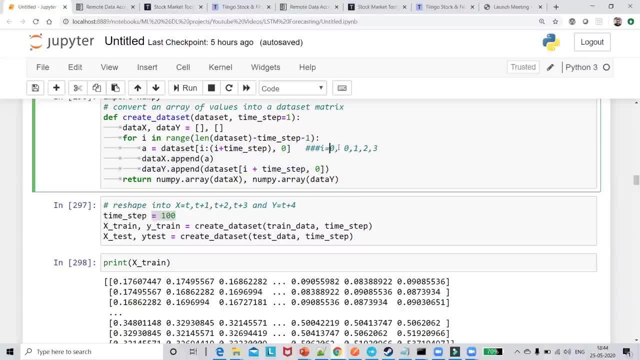 three lines code. guys. understand, in the first iteration you'll be seeing that in the 0th iteration 0, 1, 2, 3 elements will be going as your first record and your third element will be actually fourth element will actually be put up in the X if your timestamp is 3, if your timestamp is 100, like this it will be. 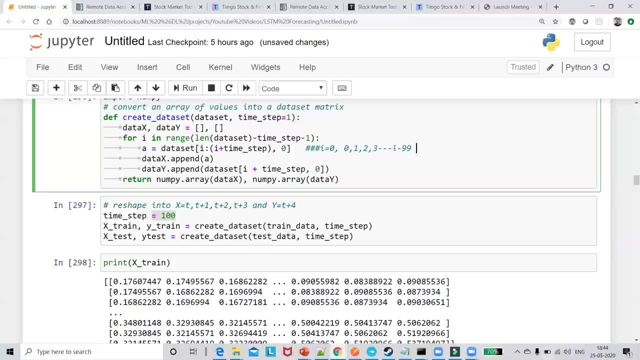 happening for 99 elements and then this will be in your extreme first record and in your white rain you will be having your hundred every right. similarly, in the next record again, you will be starting from first element till 100 element, and 101 element will be going in your y-axis. so if you consider this, 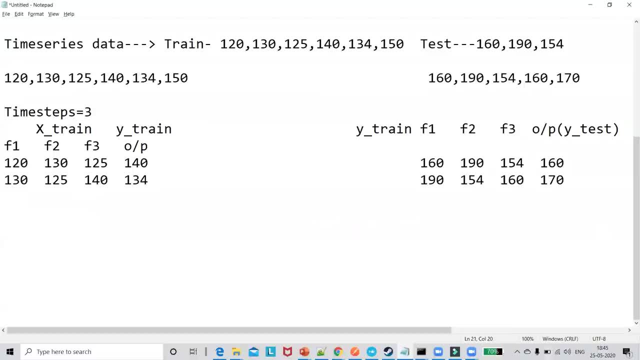 particular example. I can consider like this: let's see, so in the first f1 it will be like how many features will be there somewhere around f100, right? so suppose it goes over here like 130, right? like this it will be going: all the elements and 138 element. 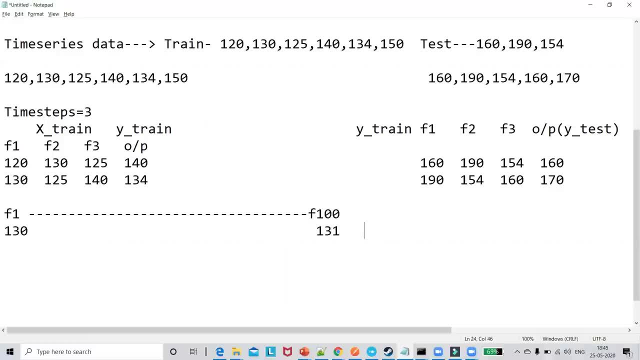 will be actually my 131, suppose I'm taking then my next element output, suppose it is 140. okay, then suppose this was my second element, like 136. okay, then what I can do is then in next record it will start from 136 and then I. 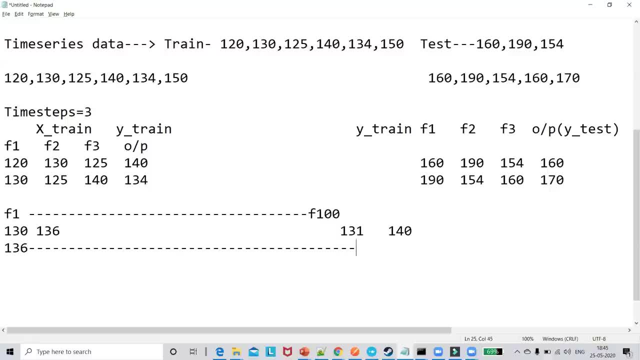 will continuously be having this output. okay, and the last element over here now will be 140. okay, and similarly, this particular element will be the next element. whatever we need to predict or we have already, we already have that particular data, so we will try to do in that particular way. 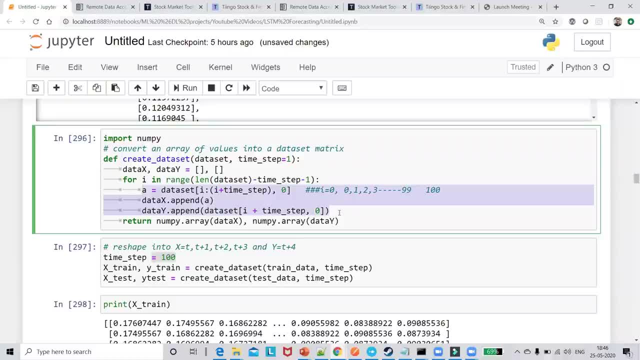 and these are the three lines of code which will actually help us to do it. okay, inside this, you can just check it out. guys, it's a very simple form of code. there right now, you will do exactly 7. let's have an hour more time. loop over here that i have written. i'm traversing through all the data sets. 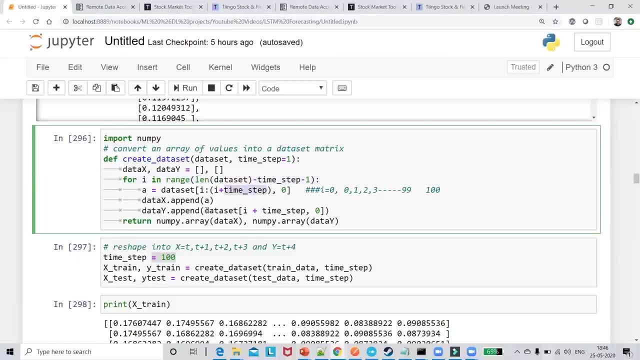 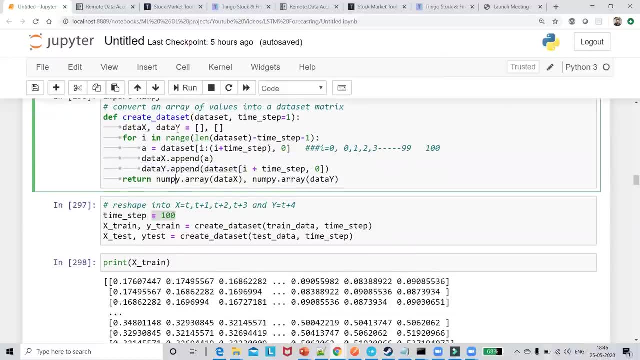 i'm making sure that, based on this particular timestamp, i'm putting that much data into my x and that much data into my y- only single data into my y, and i'm returning those values. just check this. you'll be able to understand. i'm just going to execute this. i've got executed this. 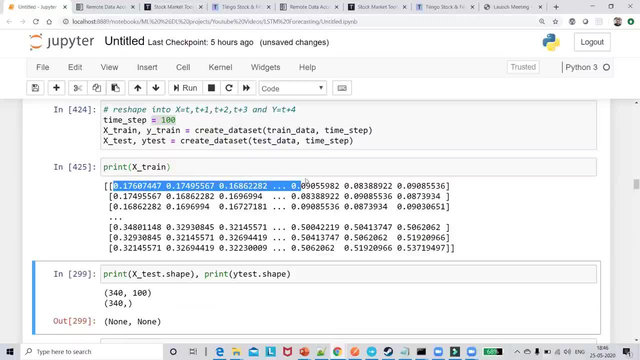 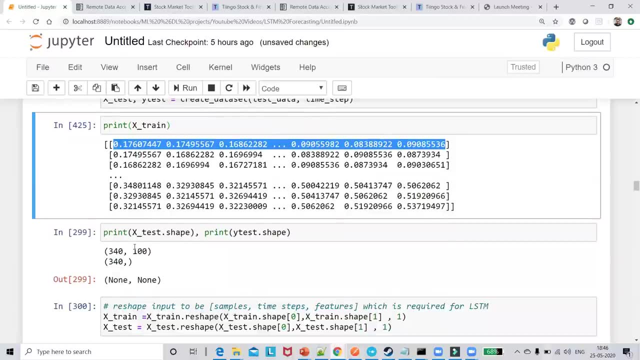 now, if you will be seeing my extreme, my per record will be having 100, uh, 100 features. you know this will be 100 features. similarly, if you can see that, you can see over here when i'm doing extreme. let me just print the shape. okay, so if i print extreme dot shape, 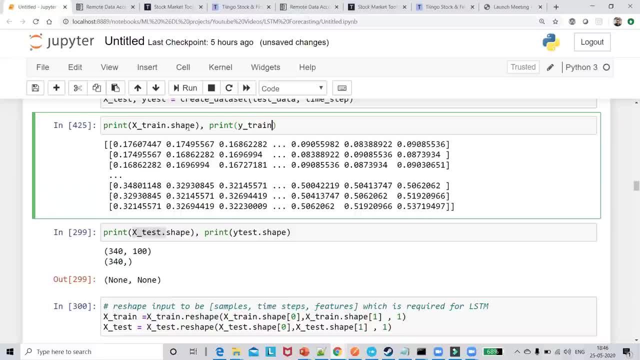 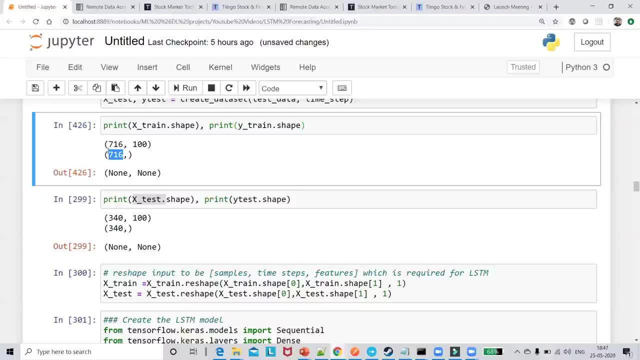 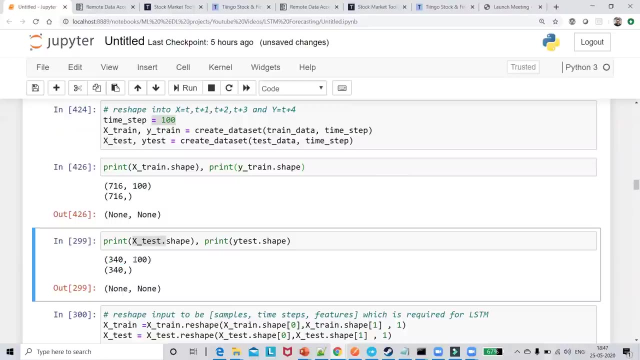 and white train dot shape, you'll be able to see that in my extreme, i have 100 features in my white train. i just have one value right and i have 716 records, so pretty much amazing. similarly, for x test, you can see i'm having 340 records and 100 features, which are same. 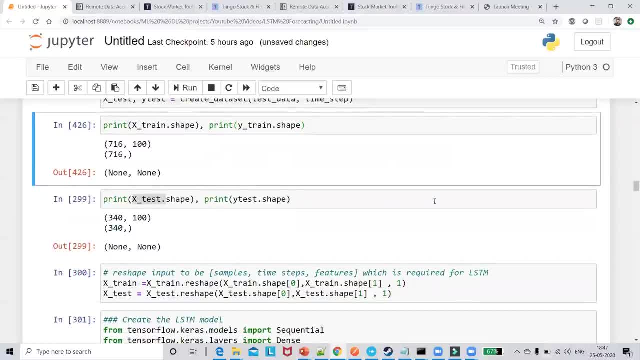 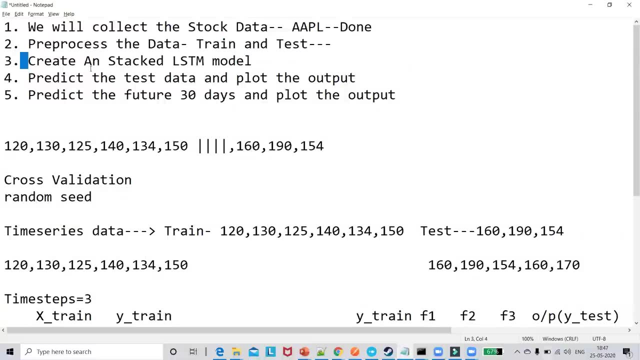 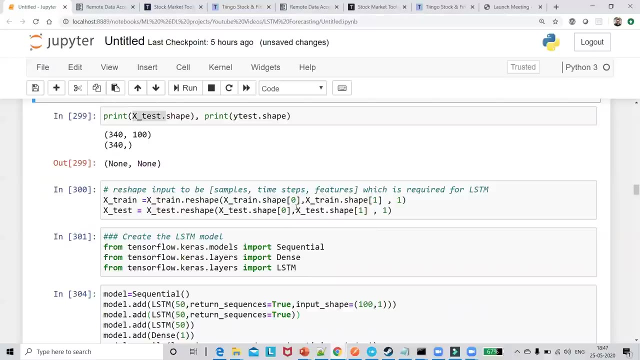 as compared to the extreme. now we have got it in a amazing way. our data set pre-processing is done. we have, we have completed basically this particular second step. now the next step is basically creating a stack lstm model. so before, uh, implementing any lstm guys, we need to always 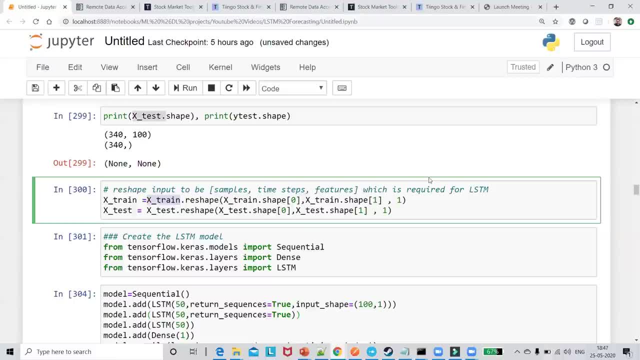 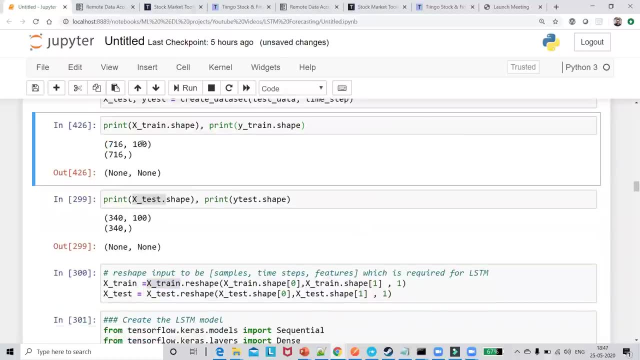 reshape our x train, you know, reshape our x train into a three dimension. now, what are dimensions are there? understand external. next steps, both. so you know that these are number of records, these are number of timestamps. there should be one more dimension which is actually converted to x. and then, if we convert this whole, 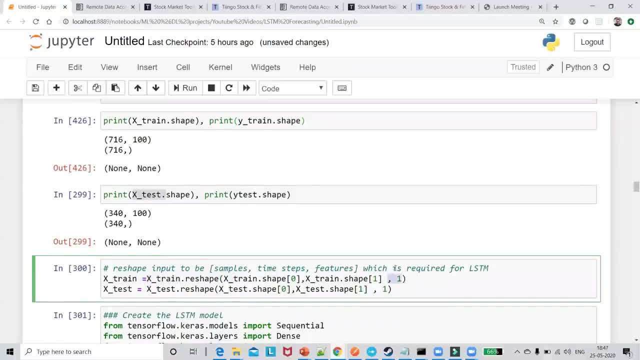 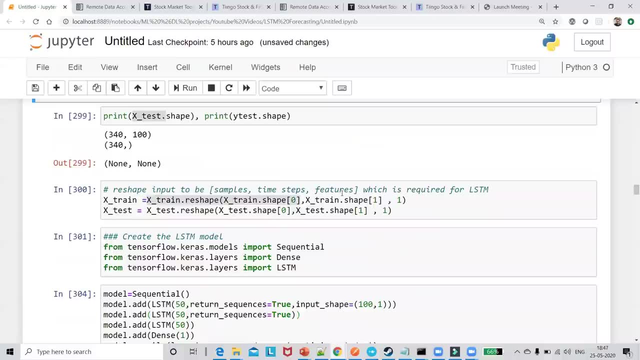 uh, shape into a three dimension. that is, basically, we need to add one- okay, one over here. so you can see that i've written x underscore train dot. reshape x train dot. shape of zero. shape of zero is nothing but 716. then x underscore train of shape of one. 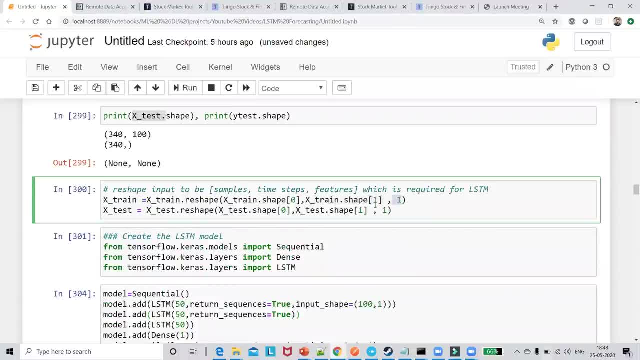 it is basically nothing but the timestamp, then this should actually be comma one, so that it gets converted into a three dimension. the reason why we are doing this is that because we will be giving this two as the input to our lsdn. if you have already. 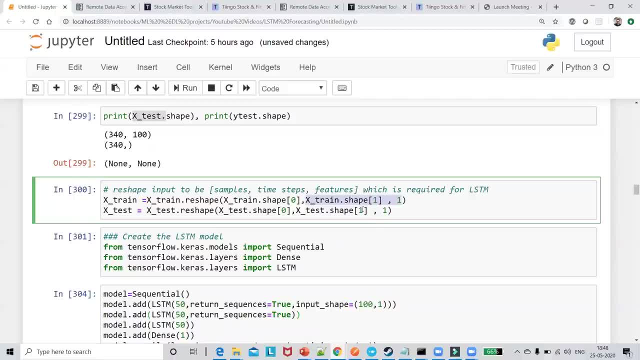 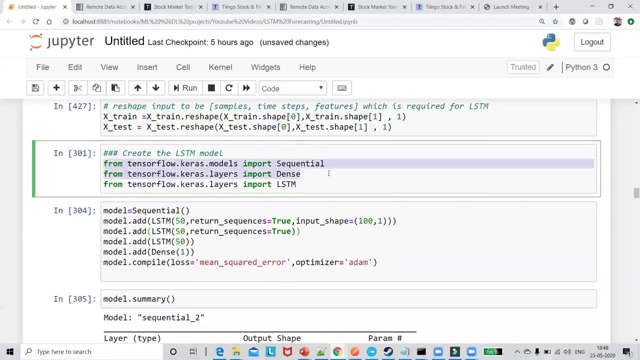 seen my lstm videos in my deep learning playlist. guys, you'll be able to understand. so this is done for the x train and x test. we have to also do it for that. then i'm going to import, i'm going to start creating my stack lstm model, right stack lsdm. so i have 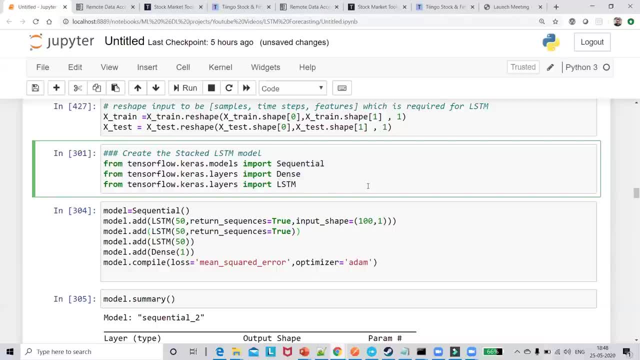 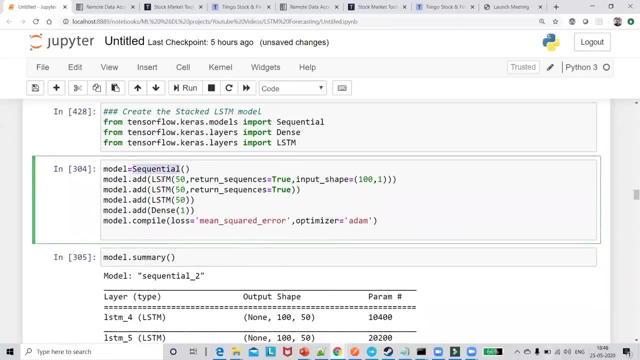 sequential dense lstm. i'm adding this: okay, these are my libraries that i'll require. lstm model is pretty much simple, guys. we will be using a sequential model. first, lstm layer: i'm adding over here, i'm giving the hidden layers at 50. i'm saying a determinative sequence is: 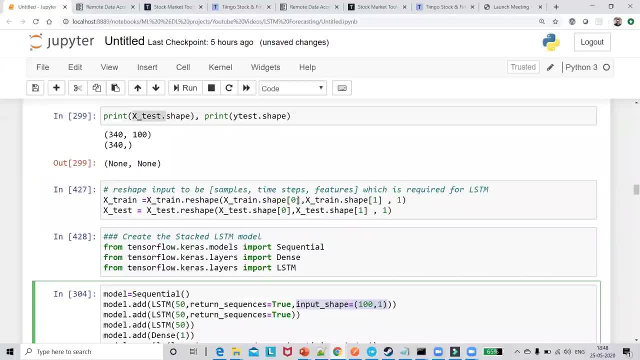 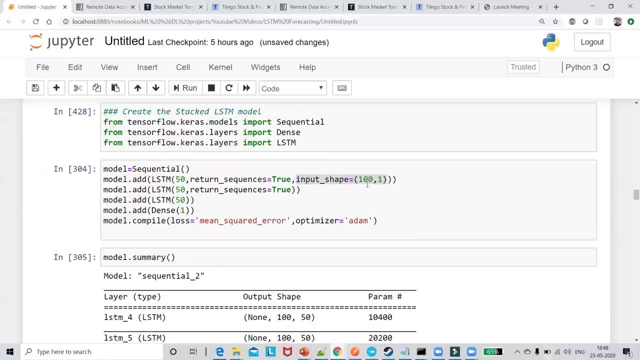 equal to true. the first input shape, as i told you should be my. this two values. now i know that x train of shape is nothing but hundred comma one, so i've given hundred comma one over here. then in my next layer i'd added lstm. uh, again, this is a stacked lstm model. 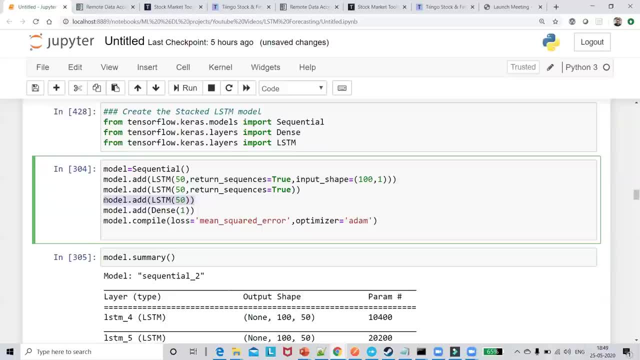 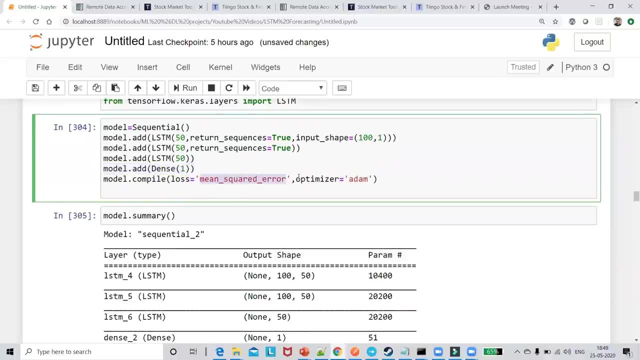 one lstm after the other right, and finally i've added one more. after that, you can see that i've added one final output, okay, and then i'm compiling with the help of mean squared error, and the optimizer is adam. okay, so once i execute this, if i go and see 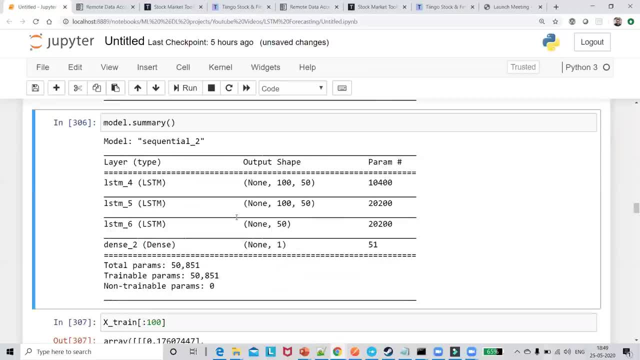 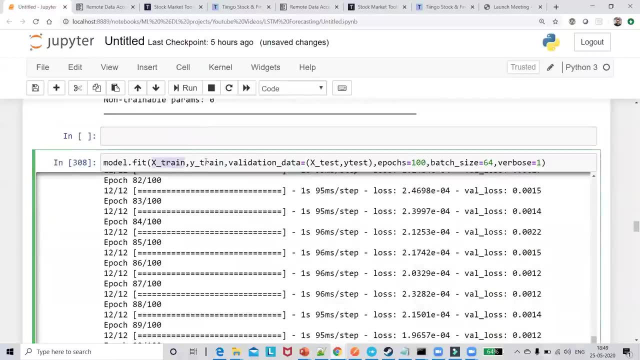 my summary. this is my summary. after that, seeing the summary, what i can do is that, guys, i'll just remove this. this is not required. i have to just fit on my x train, y train and the validation data that i'm taking is x test, y test. 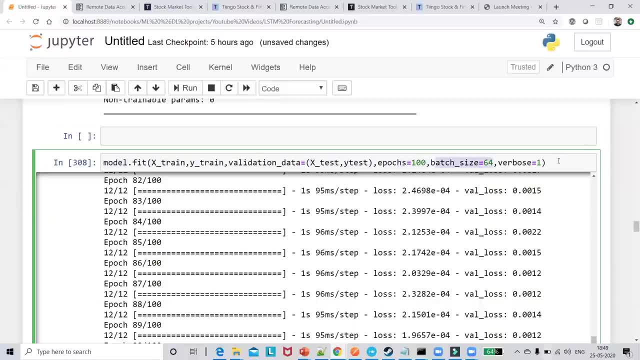 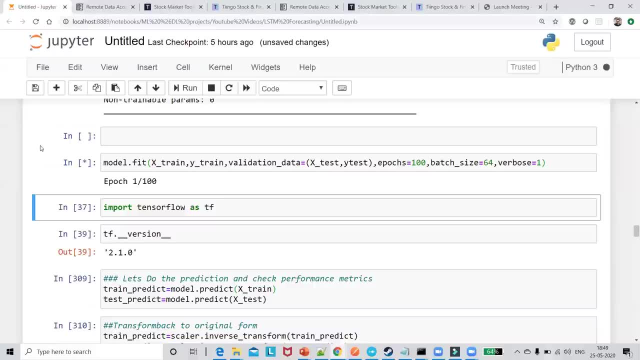 epochs. i'm considering it as 100 bath size at 64.. let me just execute it in front of you now. you, you don't have to have a gpu laptop, guys, even though you have just have i5 or i7 laptops, you will be able to. 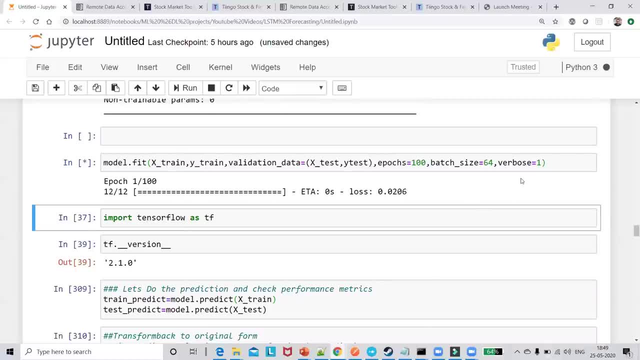 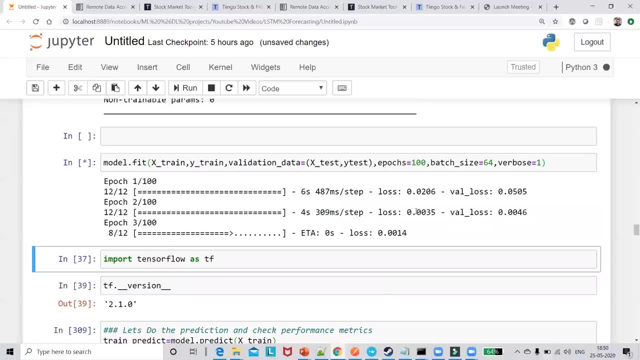 continue this particular execution. even though i have a gpu, you will be able to see that. you know i'll be able to quickly execute this. probably for me it may take one minute. for you it may take somewhere around 5 to 10 minutes if you have some. 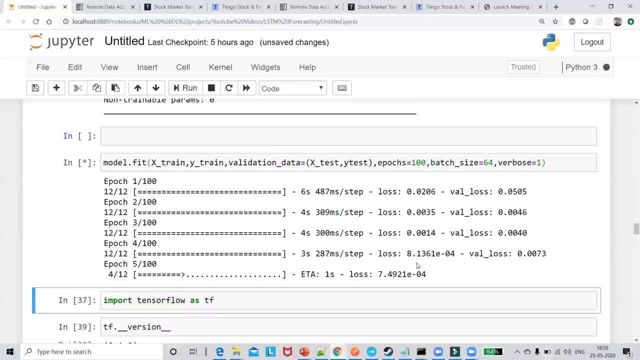 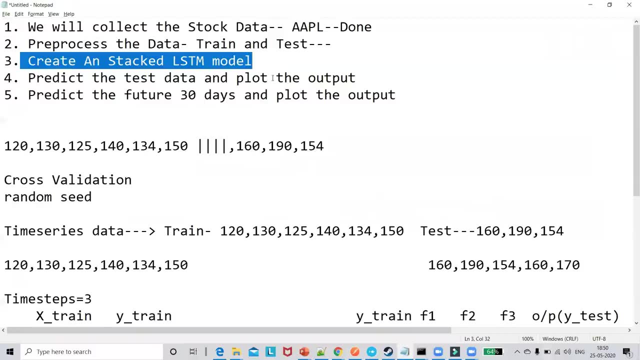 good laptop, but since i have a gpu already, it is start executing quickly. okay, so till then the execution gets over, i'm just going to go back over here, so i'm just going to provide the status over here. it is done. uh, create and stack lstm model. it is. 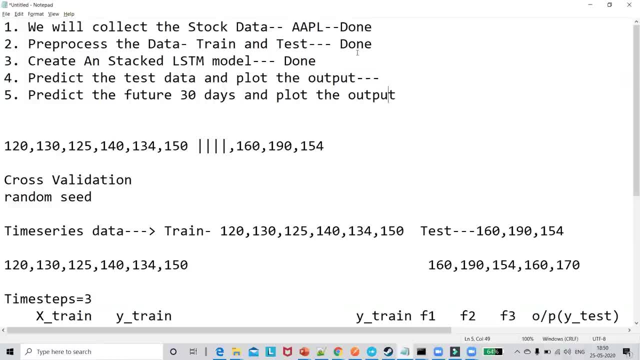 done now. this needs to be done and this needs to be done. so i'm just going to write it as in progress and remember, guys, here also, it's all about python code. what i'll suggest is that whatever logic comes up with plotting the output, it is up to you. okay, this is all about logic. you have to. 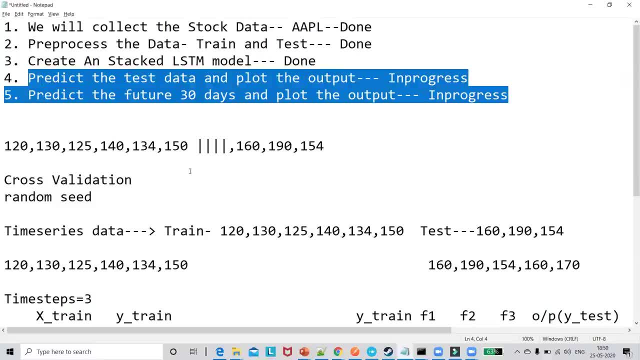 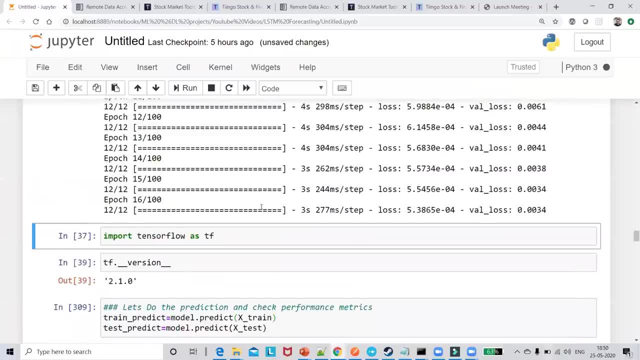 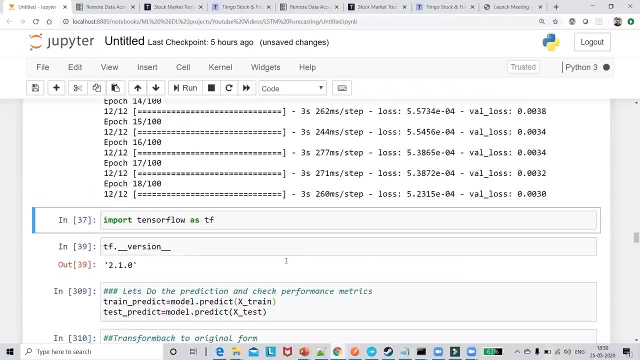 come with some specific logic in plotting the press data, you know, by using matplotlib or some other libraries. okay, so you can see how many epochs is done: 16 probably. it may take another one minute, let's see. till then, uh, we will try to explore the next line of code. 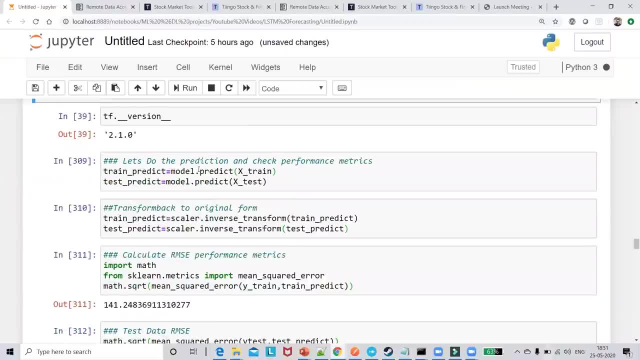 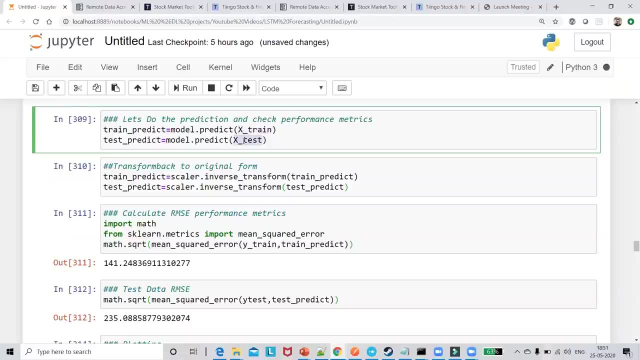 okay, now, after doing that, guys, we will try to do the prediction for the extreme data because we need to find out the performance metrics. so for extreme also, i'll be doing the predict. for x test also, i'll be doing the predict. i'll get those values. 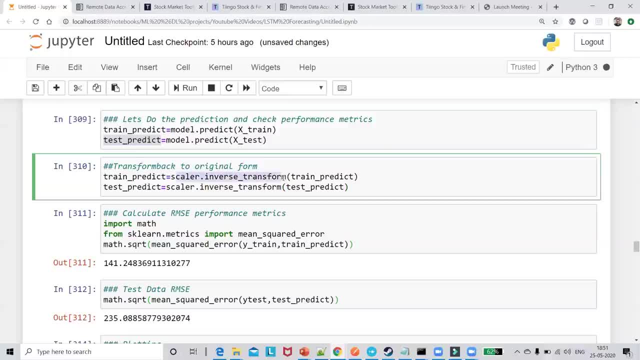 over here. then i'm also going to do the scalar inverse transform, because you understand that we have already scaled that particular. now we have to do the reverse scaling right, because i need to find out the rmsc performance matrix. the root mean squared performance. so for that i'll be using the same object, that is, scalar dot inverse. 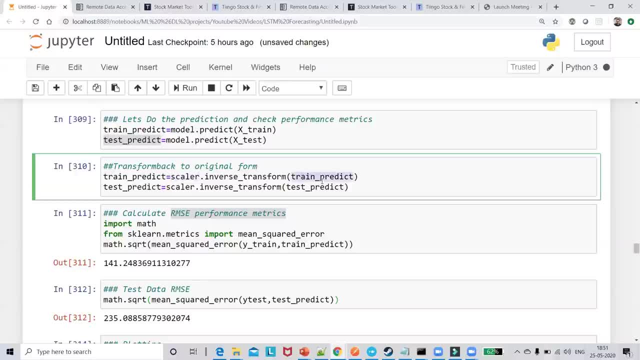 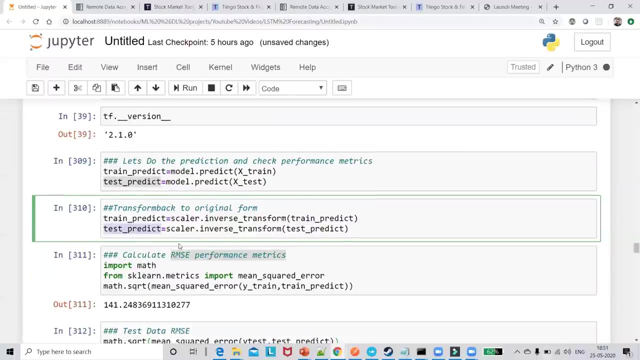 underscore transform and then i'm going to take the train underscore predict and get that particular value over here. similarly, with respect to test underscore predict, i'm going to get that value over here. right, pretty much simple over here now. the next thing is that, uh, probably, let's see. okay, 31 epochs. are there still another? 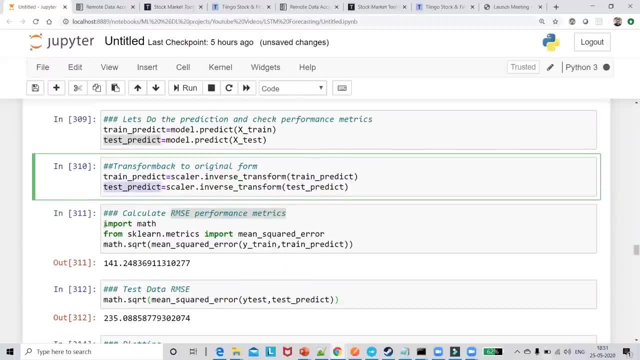 two minutes max. i guess now what we are going to do. we are going to import mac math from sklearnmetrics. we are going to import mean squared error, which is the performance matrix, and then i'm saying that we need to apply boot mean squared error. so for that i'm using mat dot. 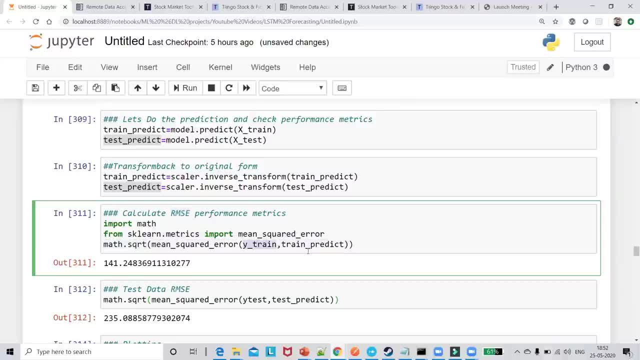 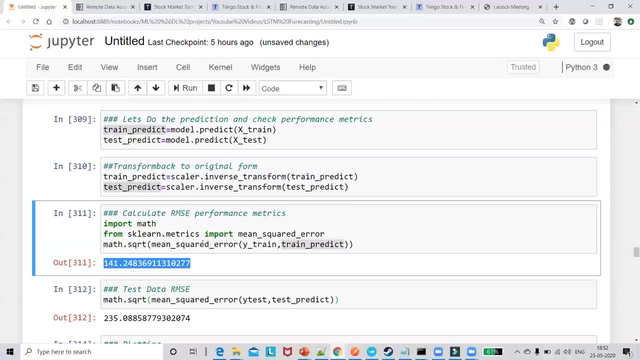 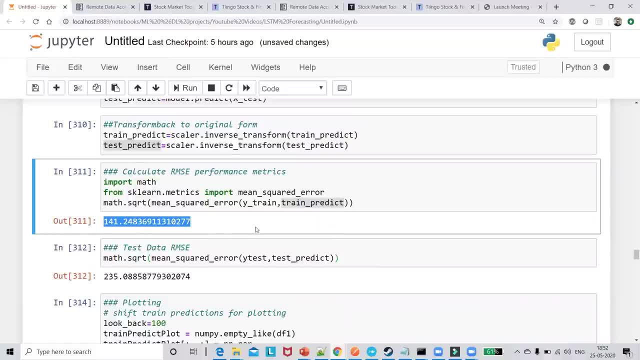 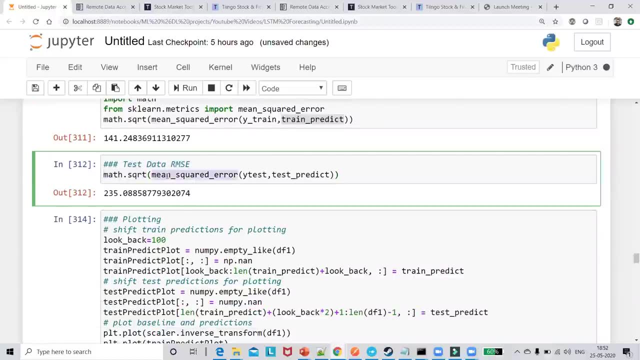 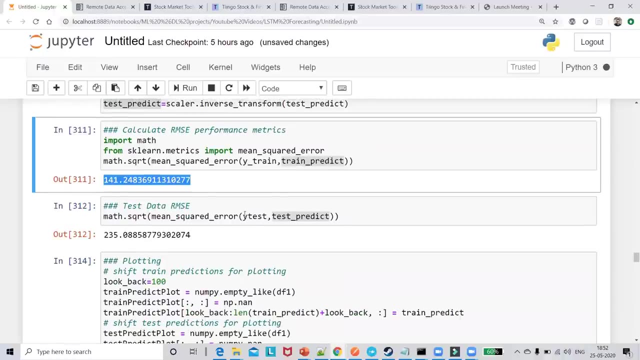 probably we can actually get a good output considering this particular value. okay now, similarly for the test data, i can again use mat dot: square root mean squared error, y test and test underscore predict. so here you can see that there will be definitely a difference, but the difference is very, very less, which is pretty much amazing. that means: 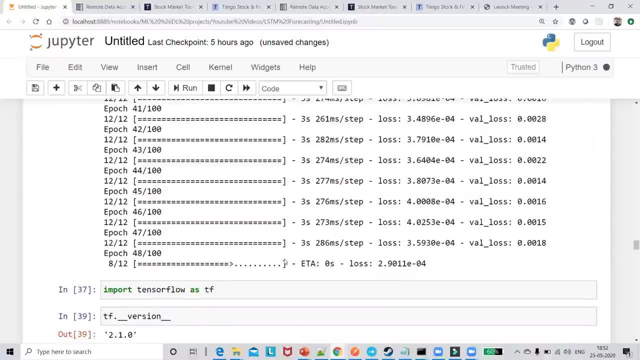 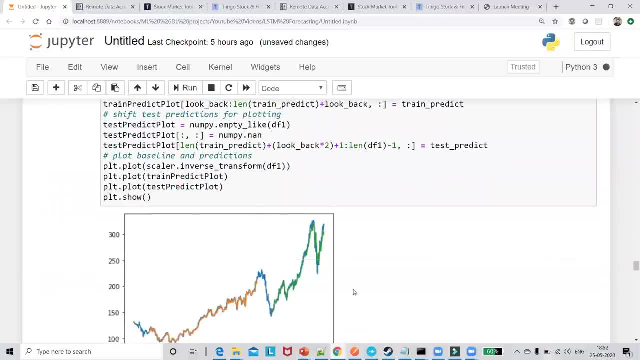 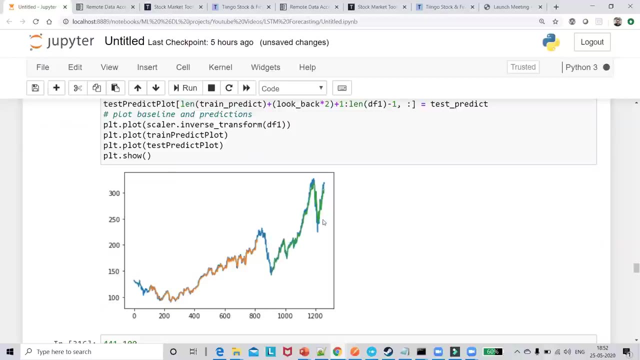 that our lsdm model has done a great work. it has done actually a good work. okay, then you can see that i'm getting a value of 235. now this is how we will be predicting, in this case, the test data predicted output that you see. that is basically my green color. 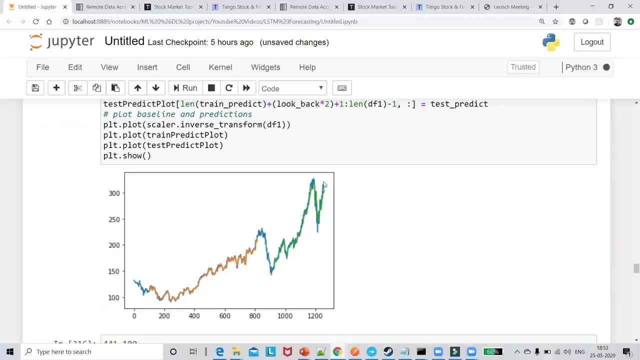 output over here. the blue color output is my complete data set, guys. uh, for the training data set that you see that what, how, how? the prediction has gone is basically this orange color. this green color is basically my. prediction is gone, basically this orange color, this green color is basically my. 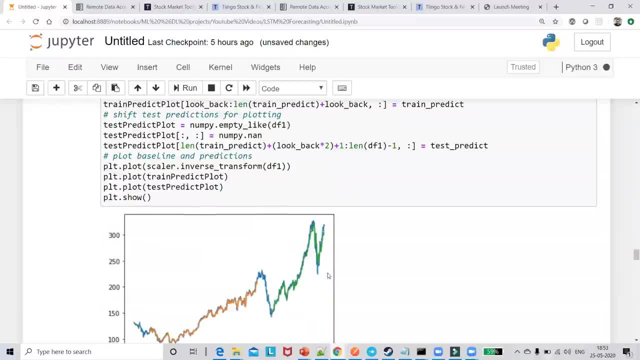 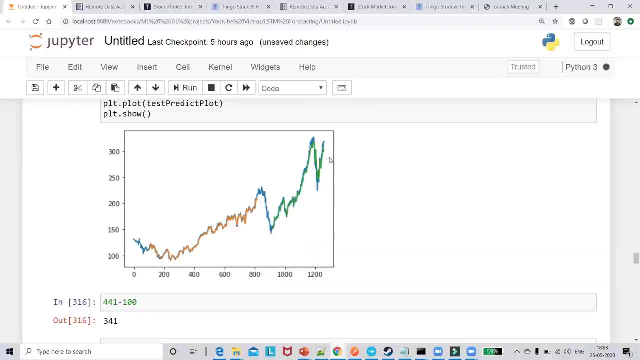 predicted output that you have actually seen for the test data. okay, so this is basically my test data, because i told you that we are going to divide the data set in such a way that my test data will be, you know, after some specific date. right, we had actually seen in this. 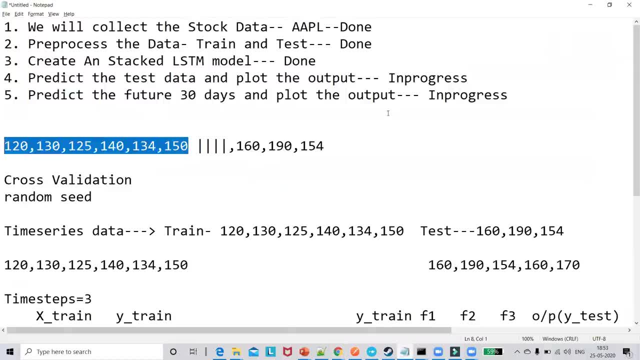 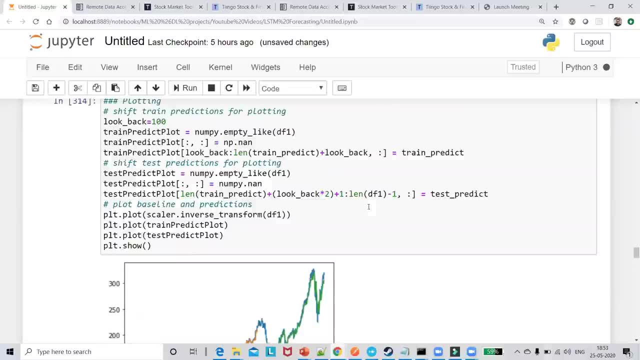 notepad right after some. so this will basically be my train and this will be my test right. so similarly, over here you can see that this green color that you see is basically my test data, you know, but still i need to do the forecasting till then. lets me see. okay, 63 ipod. 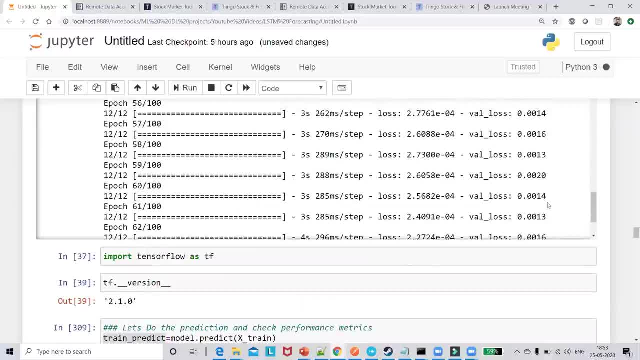 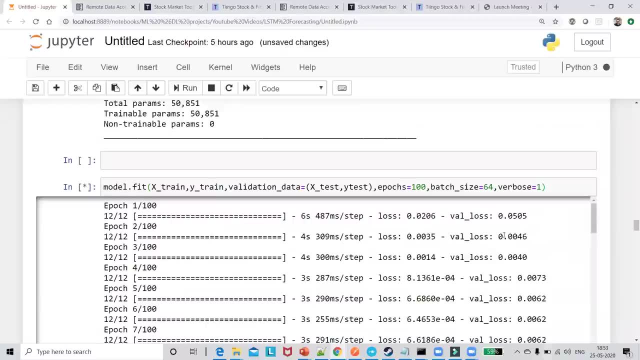 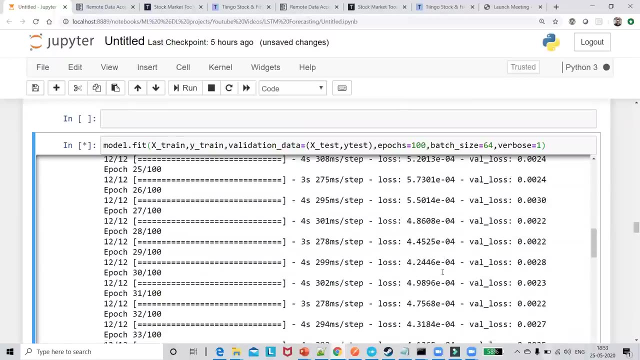 talks are done. 64, it's going on and you can observe one thing, guys: my loss value is not varying a lot now, uh, let's see from where it actually started. okay, my loss. uh, if i consider my loss, my loss had actually started from 0.02. then it is going lowering, lowering. okay, it's. 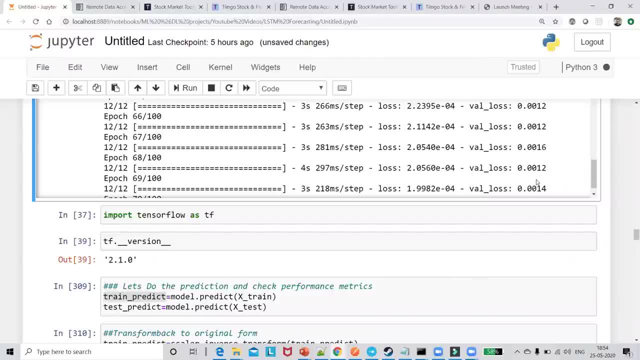 lowering in a better way. you can also see, the validation loss is also decreasing a lot. so i think we are going in the right way. we are going in the proper way because our validation loss and our loss is basically decreasing and our main aim should be that we need to minimize the loss. 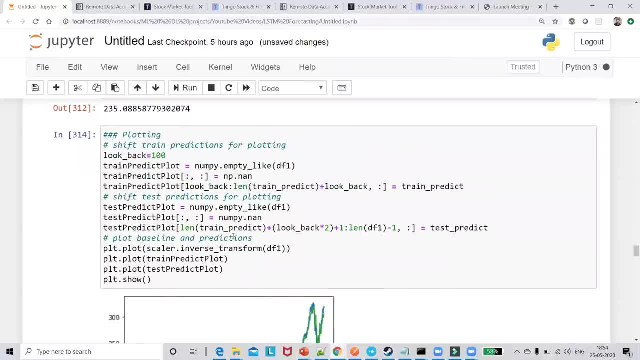 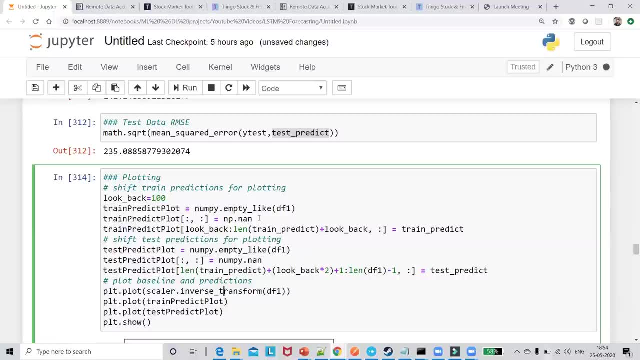 okay, now for predicting it again. uh, for plotting it. what we have to do is that, guys, we have just written this line of code, which is again pretty much simple. first of all, i'm taking nan values everywhere based on the size of the data frame. one over here. my time step is 100. okay, so considering, 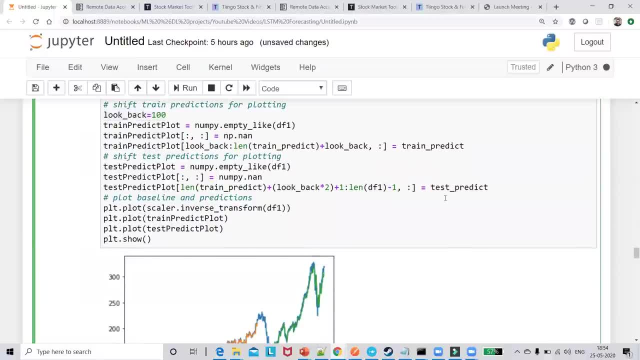 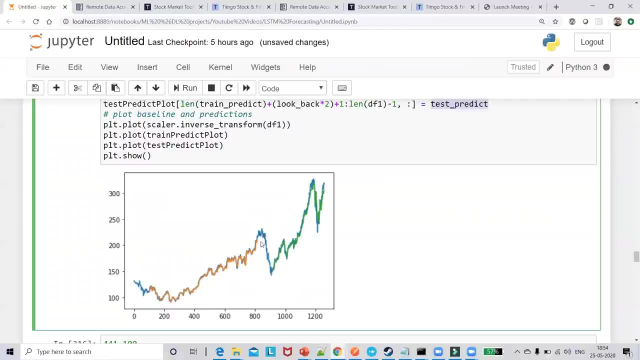 this 100. what i'm going to do is that whatever train predict and test predict i've got, i'm just plotting it over here. okay, i'm just plotting it. this all data that you see till here is basically my train predict data and this is my test predict and before that, always remember: 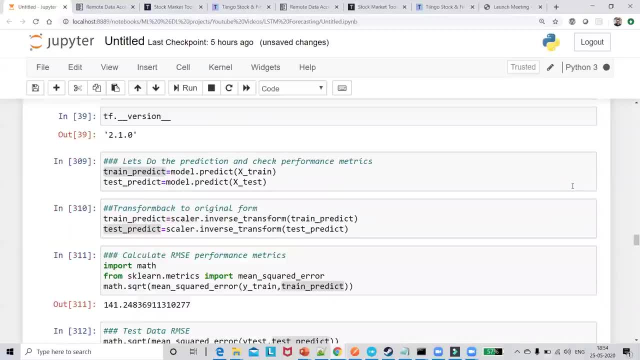 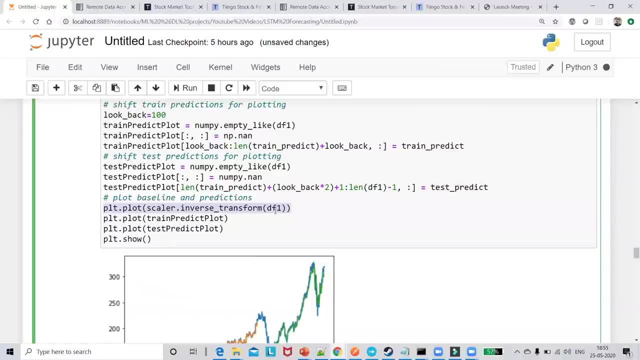 you need to do the scalar dot inverse transform, or don't forget about that, guys. you always have to do that, otherwise you'll not be able to get it in a proper way. so, df1, you have to do this, this two. already you can see that test underscore predict and train underscore predict. i've already. 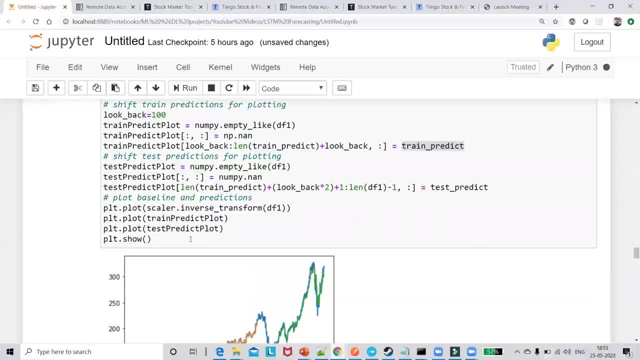 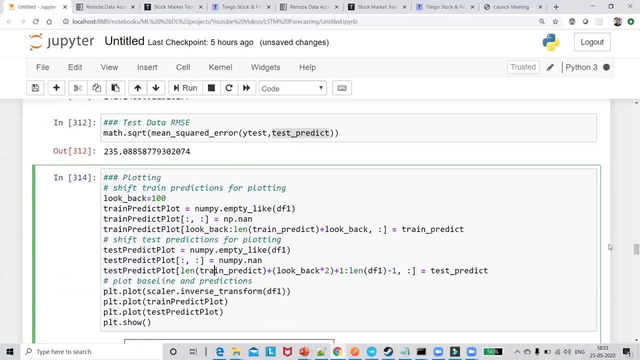 done the scalar dot inverse transform. this is pretty much simple code. just try to have a look. it will just uh, you'll be able to understand it. just download it. i'll have given you the code in the github repository, so i hope, uh, okay, 92, 93. 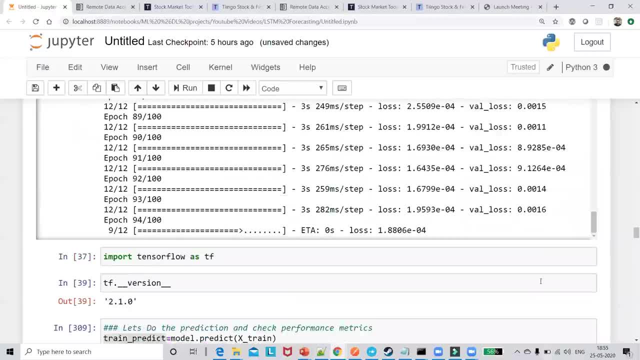 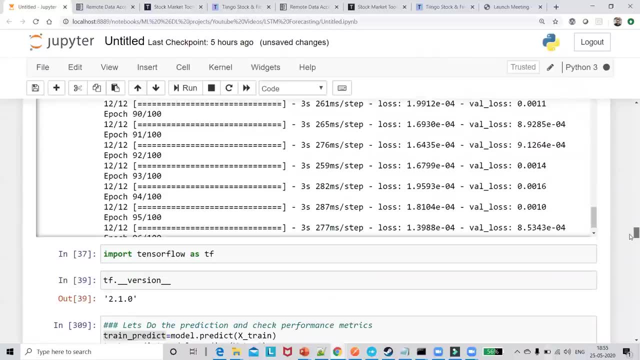 94, but it's, it's, it's good, you know it's. i feel good that i'm actually working in my laptop and quickly i'm able to train it. i'm able to explore a lot of things from when i've actually bought it and i'm able to train it and i'm able to explore a lot of things. 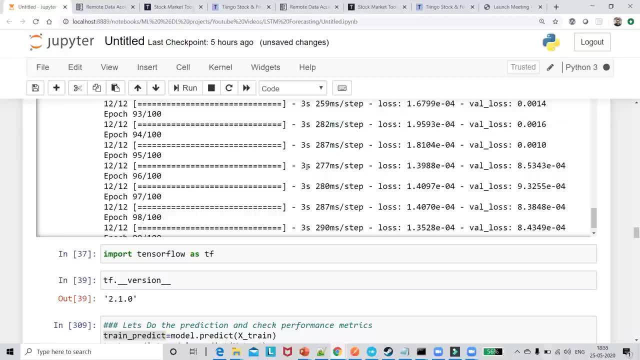 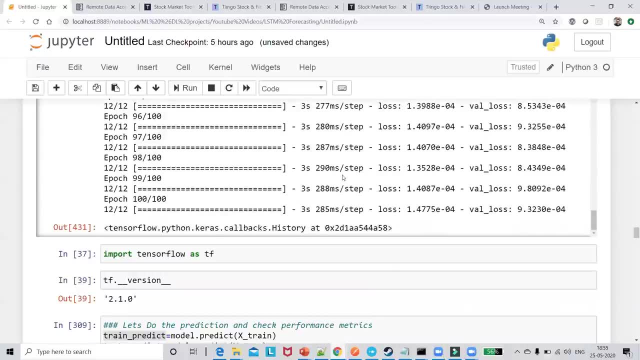 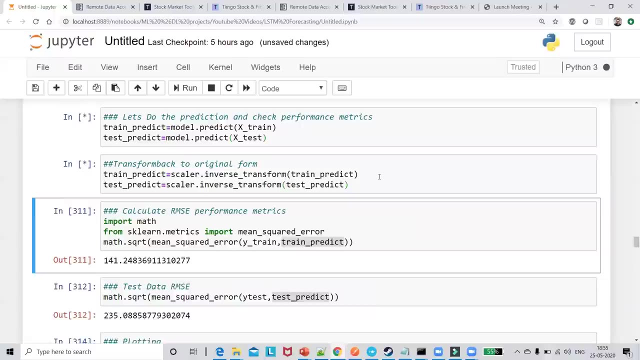 from when i've actually bought this laptop. you know i'm able to do a lot of work actually. so, yes, uh, last epoch done, okay, perfect, so this epochs have done. now i'm just going to do this execution, execution, oh, probably it's taking time, okay, done. this is my oh. it has got reduced. and then the previous value. 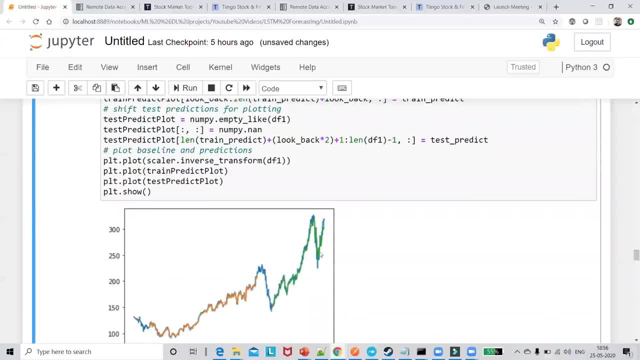 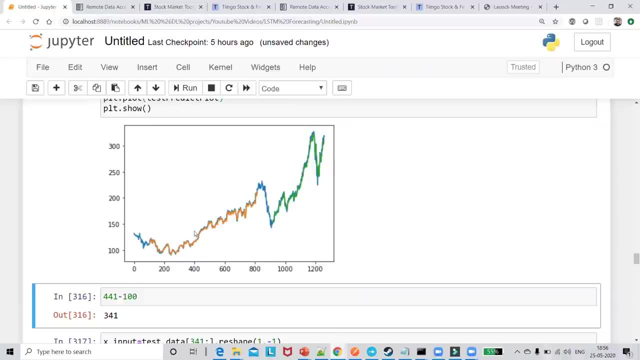 okay, this is 235, which is almost same. now, we will be plotting this. you know we'll be plotting this. this is my test data output that I have predicted, considering this green line, this orange line, is for the train data. now, remember one thing: what we have to. 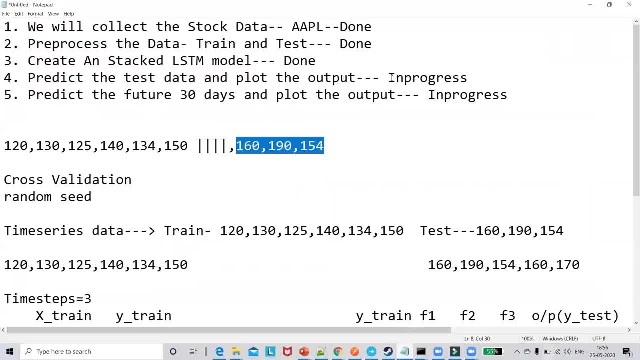 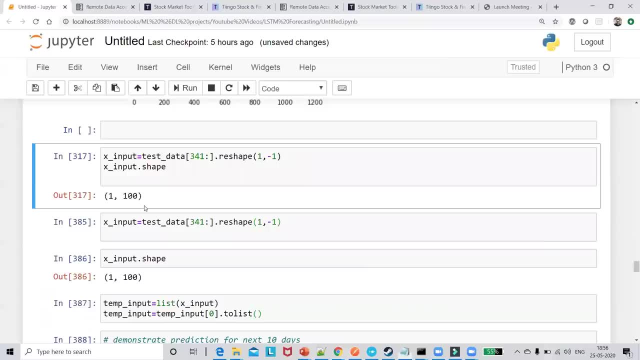 do. now the next step. I told you that we have predicted the output and this is done. okay, so this is actually done. now, predict the future 30 days. okay, guys. and for this, again, I had to write a lot of logic. understand that if I go and see my 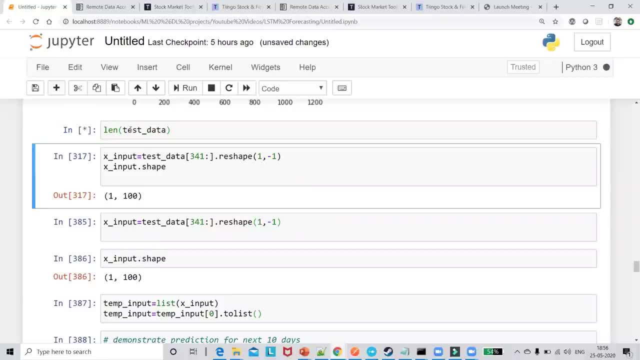 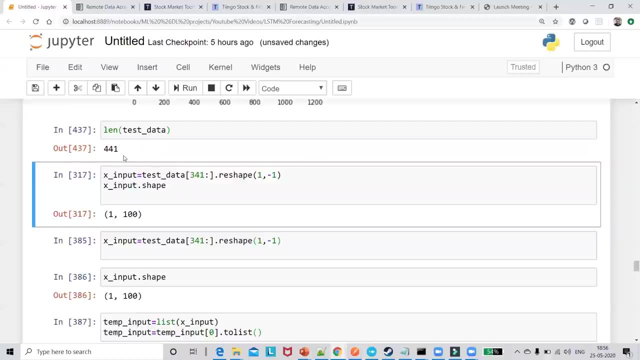 length of test: underscore data guys. it is 441 441 record, so I have to. actually I wanted to start from if I consider: okay, suppose I consider that in my test data my last date is somewhere around 20, 5th, 22nd me, okay. 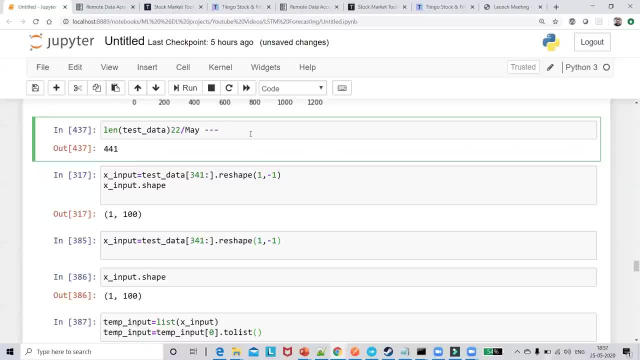 now, to calculate the output of 23rd mean I have to take the previous hundred days data Right. Then only I'll be able to predict my 23rd May data or output, you know, by giving it to my LSTM model. So it's the same thing that I am doing over here. Over here you can see that what I am doing, I'm taking from 341, 341 to 441 data. 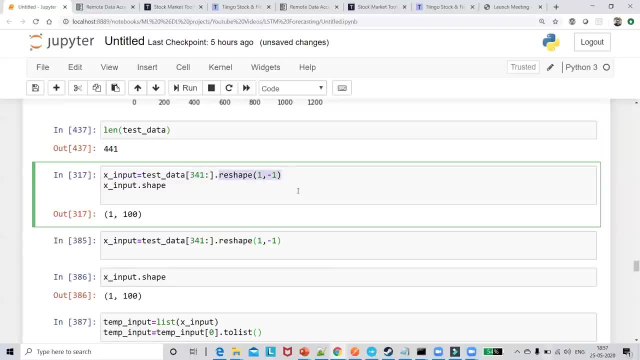 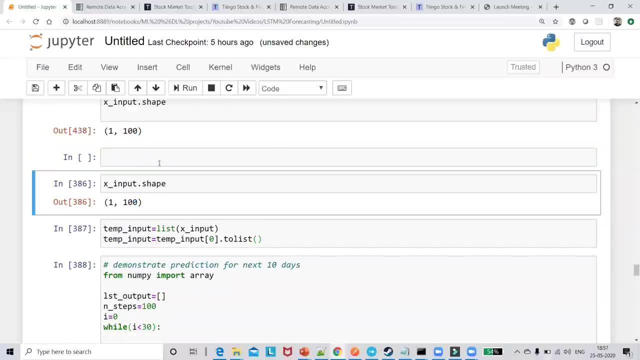 That is my previous 100 days, And I'm reshaping that into one comma minus one. So once I do it, you'll be able to see that I'm having 100 data over here. OK, so this is also the same step. I'm just going to remove this. I'm going to remove this. 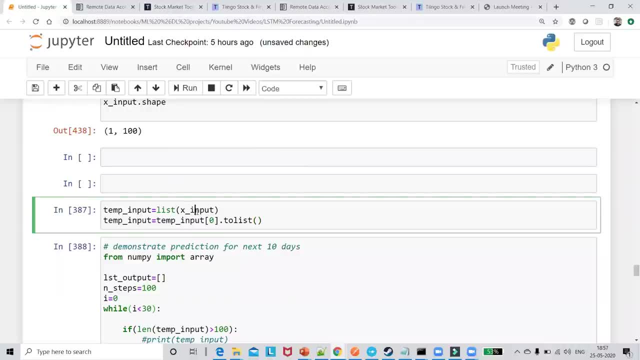 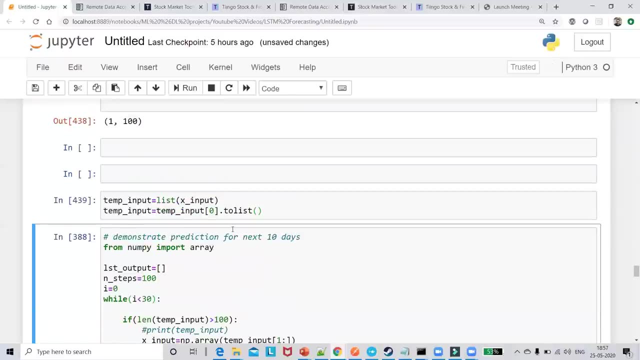 OK, now, after this, what I'm going to do is that I'm going to convert that into a list. OK, list, I'm converting it and I'm actually taking all the values from there. So once I execute this, Let's see my temp underscore input. 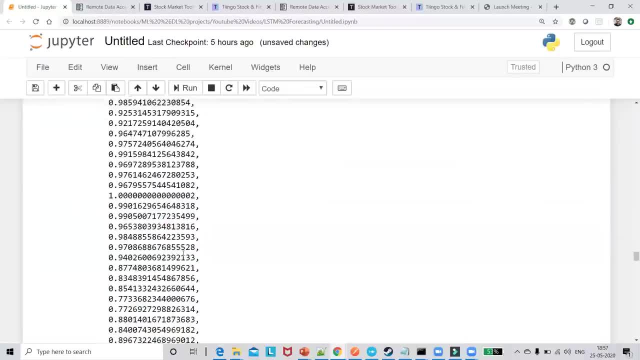 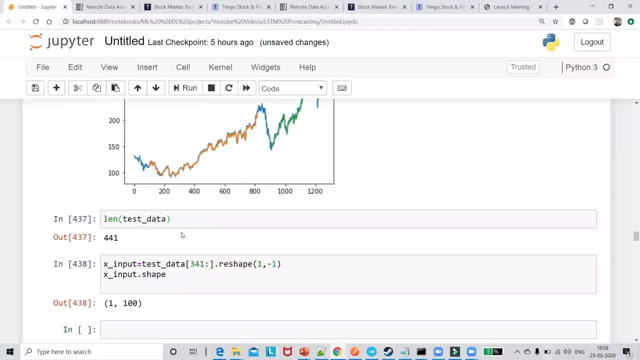 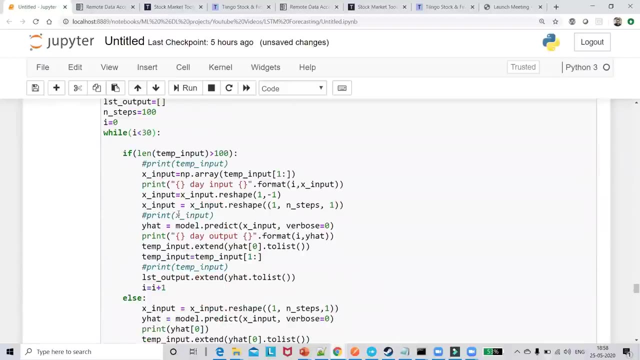 Temp underscore input is basically all my values. all my values you can see over here. That is basically all my data from this test underscore data. I dissolve all my test underscore data values, The previous 100.. This is 100 data. OK, and then I have actually done a logic. 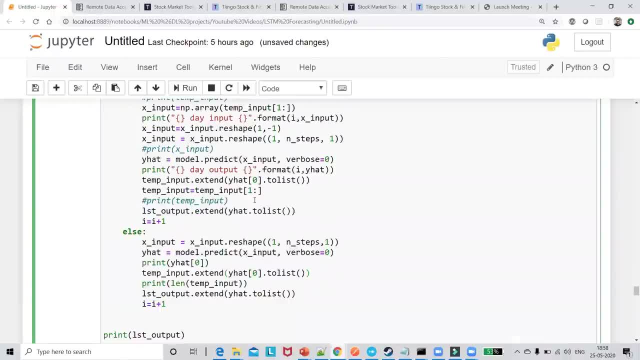 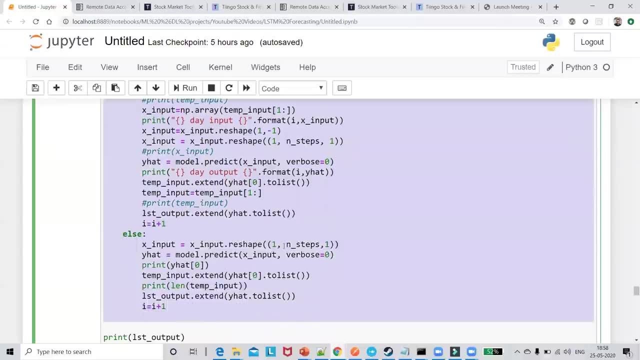 A logic, basically to find out the next 30 days. You can see that I've written a condition. Well, I is less than 30. I have to run this particular loops in the first. This will go inside this. OK, so what is happening? Let me just tell you what is happening inside this. 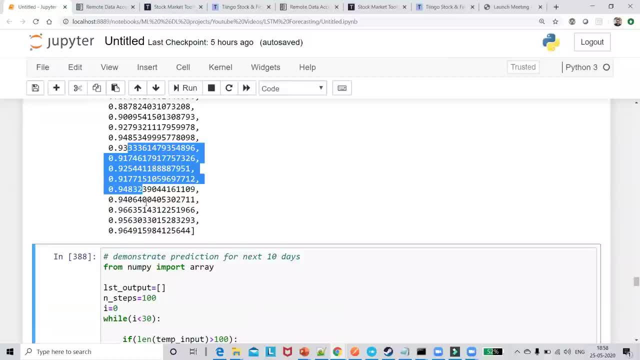 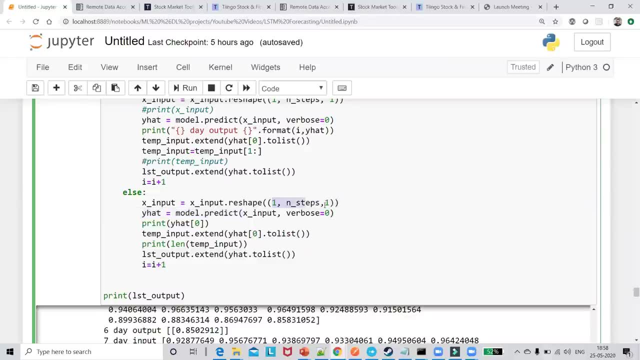 OK, inside this, what we are doing is that, whatever this 100 results we are given, we are passing it to our model and we are doing The predict, And before that, we need to do this reshape that we always used to do right in LSTM. 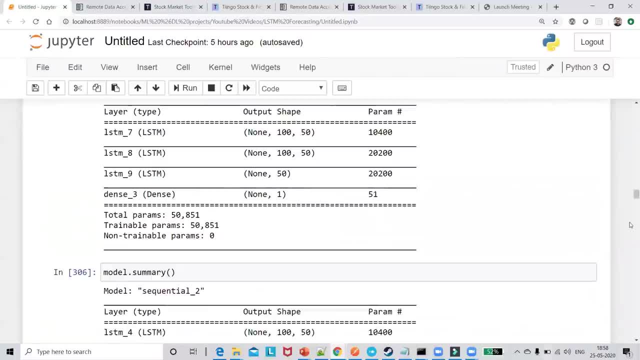 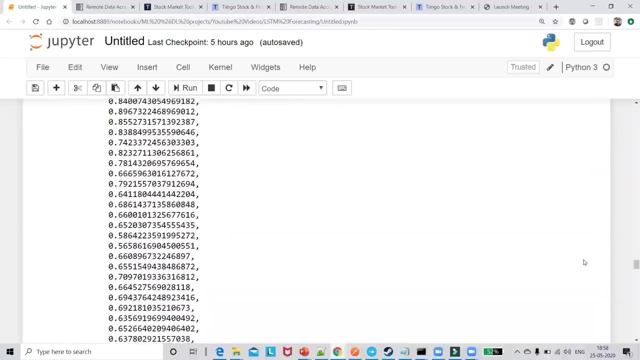 You can see that. I told you that the first step is always doing the reshape right. So here also we have done that reshape. So for the new data also, we always have to do this reshape, So this reshape. you can see that we have done over here. 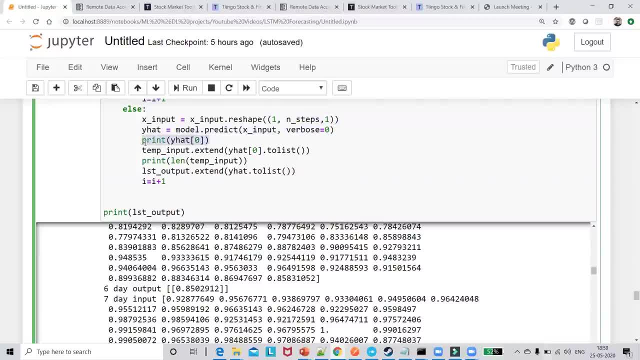 Then we are doing the prediction. I'm getting the y hat value. I'm adding this y hat value inside my final output. OK, well, here you can see that I'm adding it. And then I'm also adding it in my previous input, in my previous input. 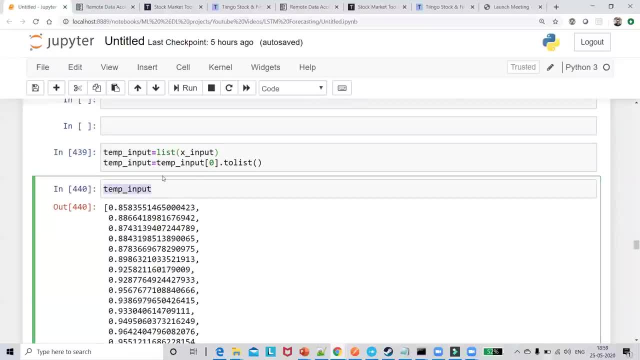 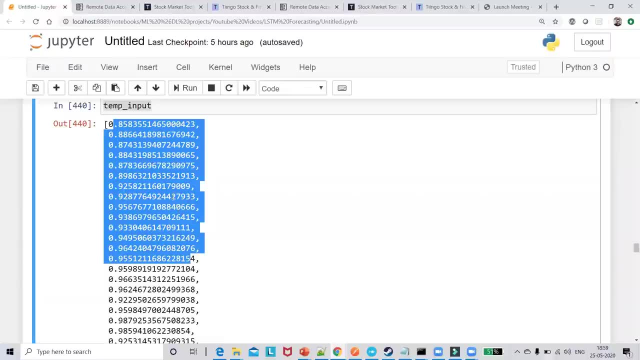 which input this particular input? guys, whatever input I had in my data set right, This is having 100 data. Now, when I add into this particular list, it will now have 101 elements. Now I have to actually shift from one position and take the remaining data. 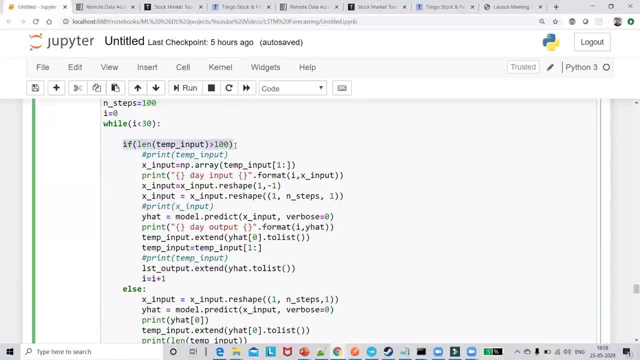 And that is what. that is what I'm actually doing. inside this condition, I'm saying that if length of temporary temp underscore input is greater than 100, I'm going to take from the one position that basically I'm shifting one position to the right and I'm taking the new output as 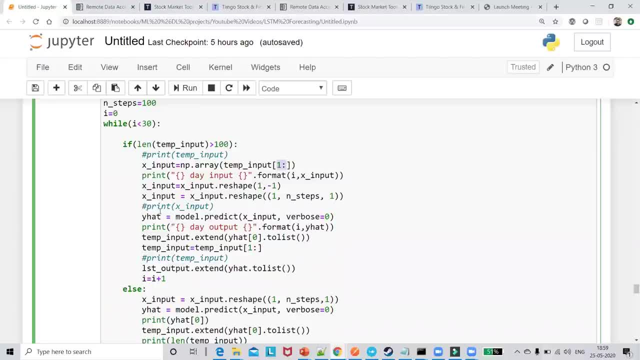 and putting that into my input, right? So I'm doing that same steps over here and doing it reshape again, and I'm doing the predict And finally, again, this will condition will be going on unless and until we complete 30 loops and probably we'll be getting this particular value in that specific 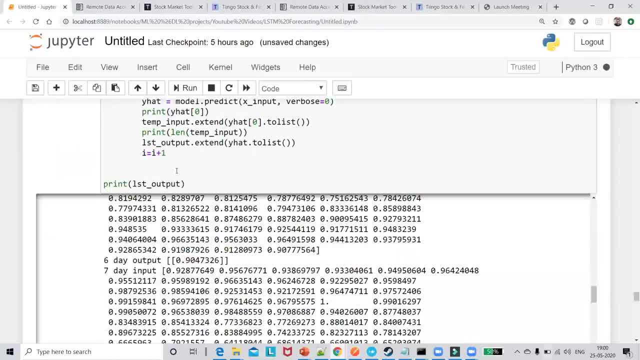 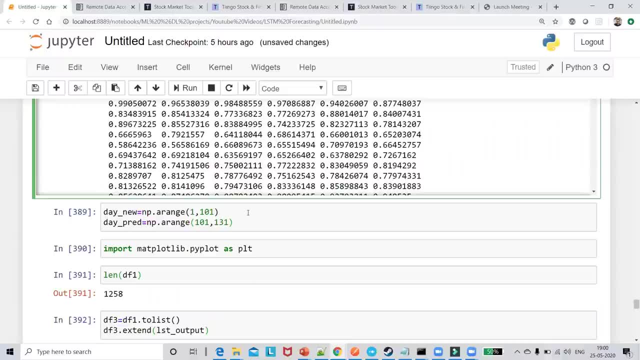 way. Finally, once I execute it, you guys, I'll be getting all the output. I'll be getting all the output inside this list, underscore output. Then now the thing comes is, with respect to the plotting, how we can actually plot. 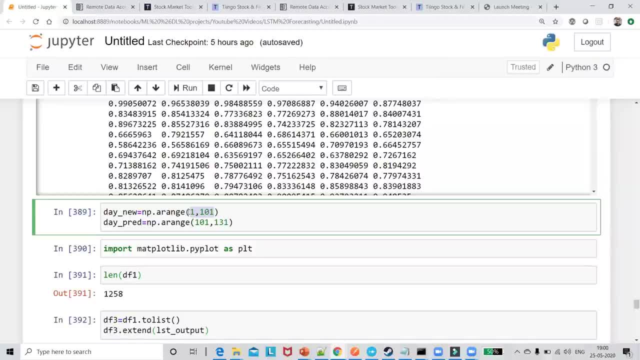 So you know that for my test data I've taken the previous 100 days. So I've kept a hundred indexes inside this day underscore new. In the predicted underscore day I've taken 101 to 131 because 30 days future I need to. 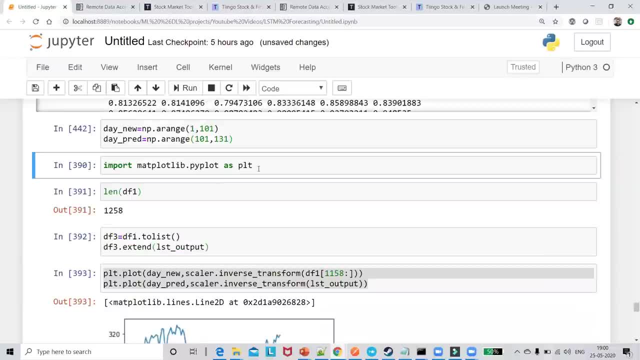 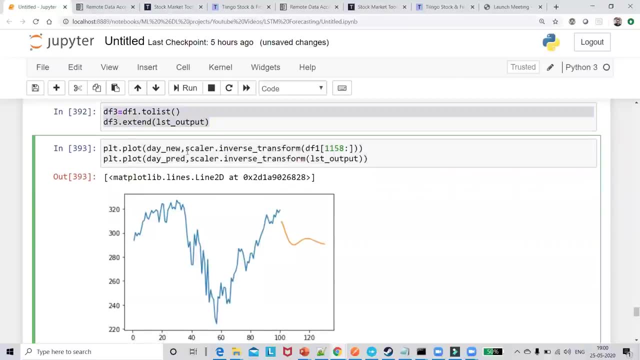 predict right. So this will actually come in my x-axis. I'm going to use matplotlib. I'll come to. this particular thing is just a second. So I'm saying: PLT, dot, plot, scalar, dot, inverse, transform, BF. one of one, one five eight. 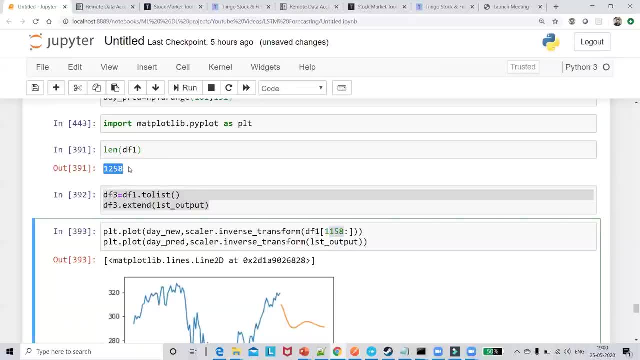 Now why I'm saying BF: one of one, one, five, eight. Understand guys. the total length of the F1 is one to five And I've told you that I've taken the previous hundred data. Right, I've taken the previous hundred data. 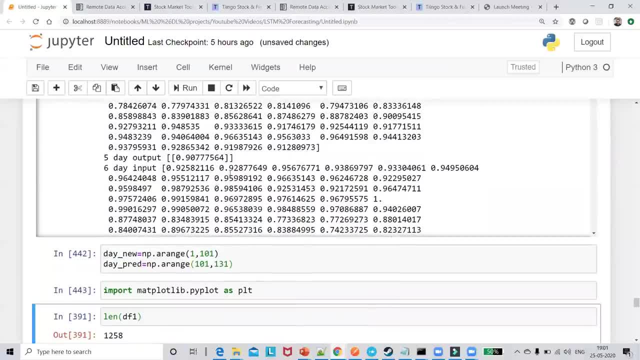 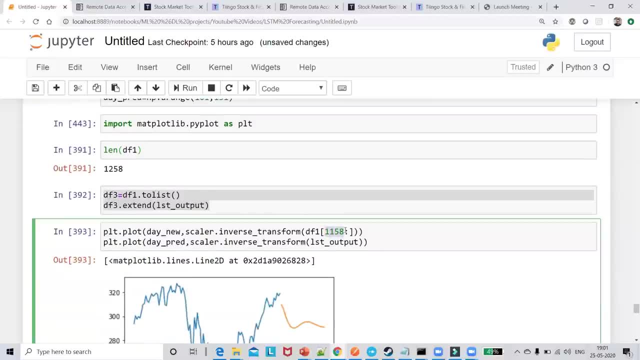 So when I'm taking the previous hundred data to do the future prediction over here, so this hundred data will be having the previous hundred data itself. So I'm saying that from one one five eight to one to five eight. you display that as my real. 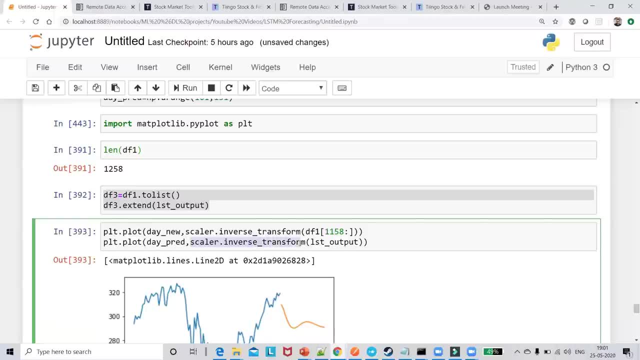 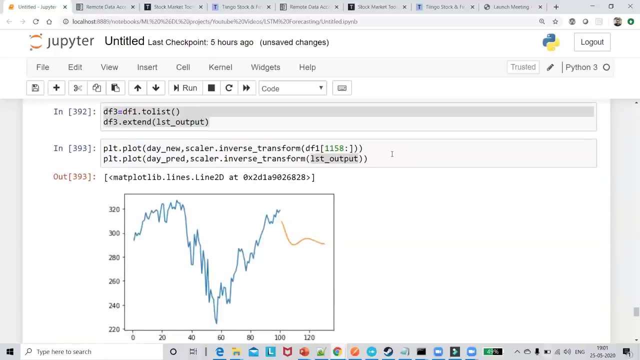 data. Now my predicted data will be: scalar, dot, inverse, transform list underscore output. This list underscore output is basically: I'm adding all the output inside this Right. So when I do this, you will be able to see we are getting a wonderful graph which looks: 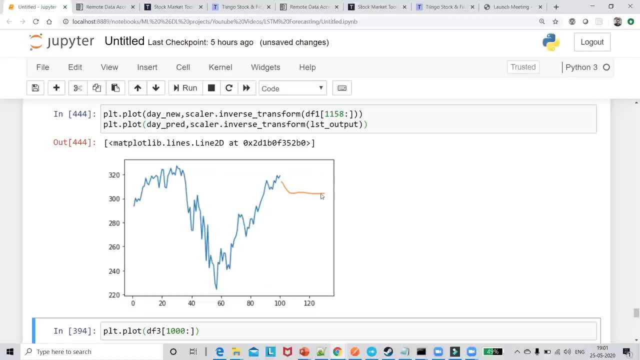 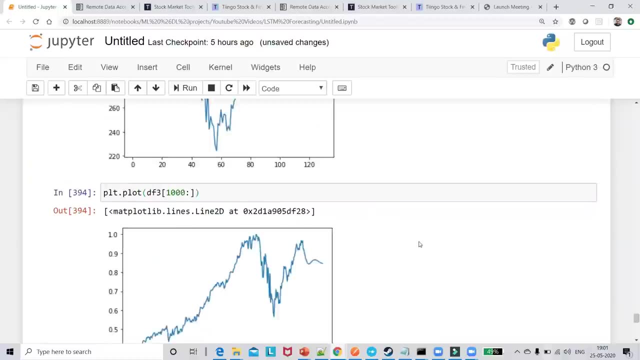 like this: OK, this is the new 30 days output that you can see And I think You have done wonderful work. OK, but still, if you want to see the complete output, I would suggest is that just try to do in this. 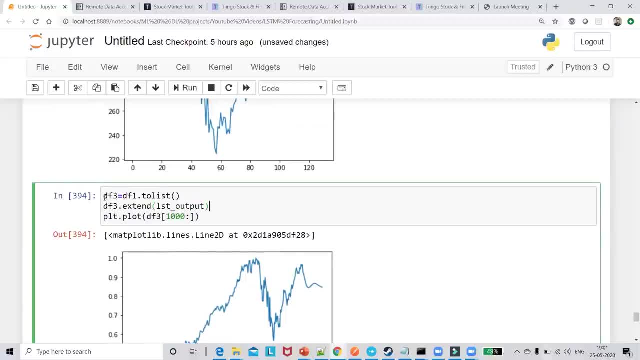 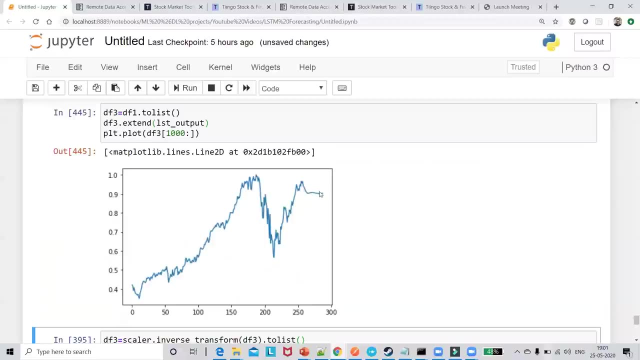 particular way. combine, combine your DF one and your list output inside BF three and just try to see how the prediction comes. Now you can see that at the end. this is my 30 day and it will be actually smooth and you know. 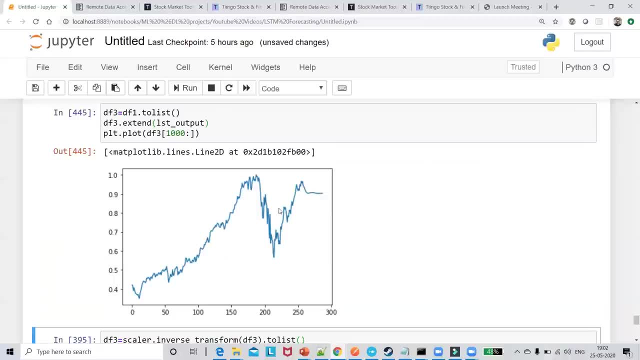 and compared to this exact way, we had this particular stock price. it is actually smooth and you can see that it is also Going up and down. If you want to really see in a proper way, just start from twelve hundred. Now here you can see that how this data is. 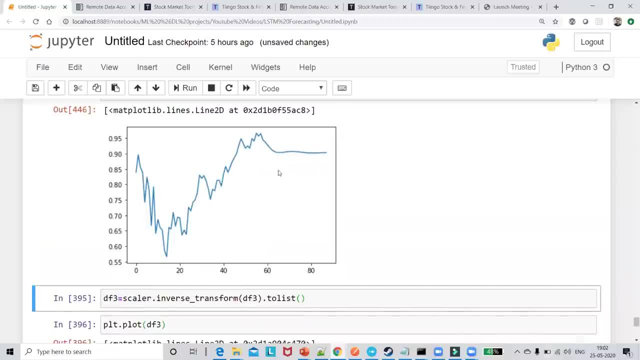 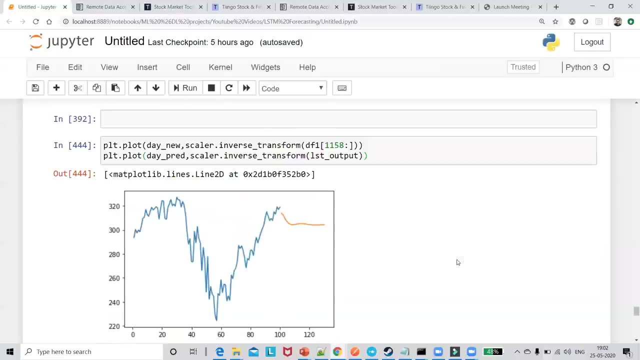 And here you have a good visible visibility with respect to this particular point of fact, like how the data or the stock price is predicted. So I hope you have understood this Now, how you can improve this particular model. guys, instead of hundred, tried with one fifty times. 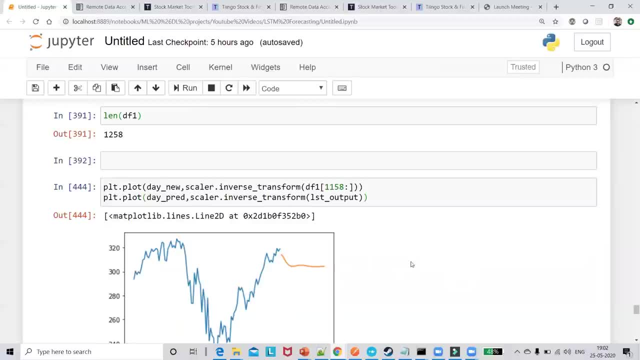 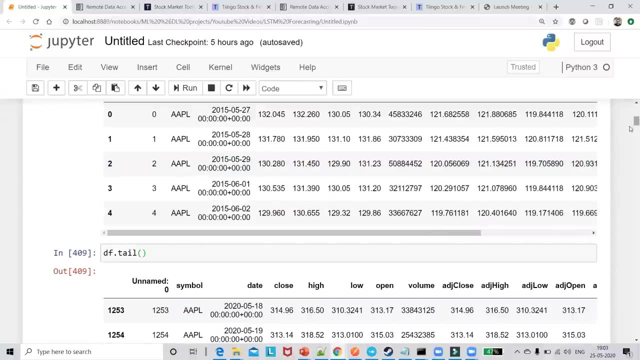 And one more thing that you can do is that try to predict for the next hundred days and try to see that How it looks, How it looks like you know, how the data, how the output looks like the video guys. I hope you are able to understand all this particular thing. 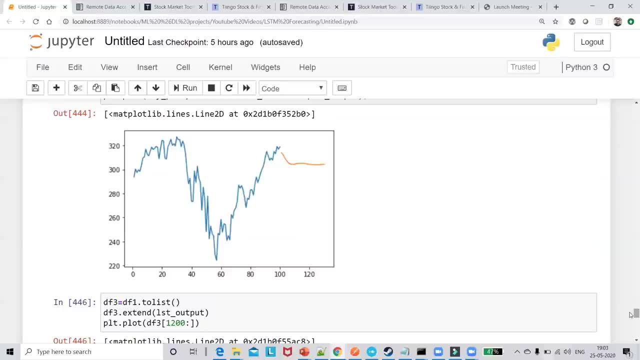 So yes, this was all about this particular video. and we can still improve the security by using bidirectional LSTM. So, yes, and that I'll be showing you in my upcoming videos. So, yes, this was all about this particular video.